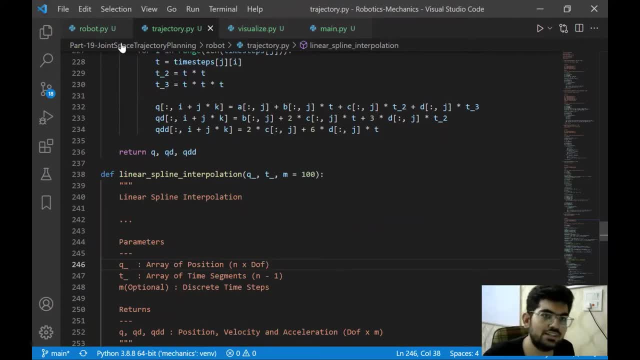 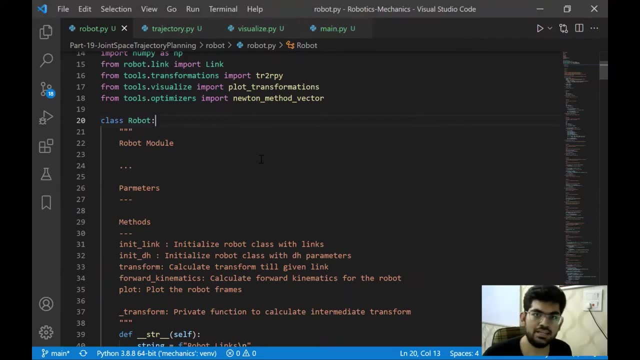 These were coded separately. We required them to be coded separately. Now we are going to implement these inside our robot class, So the trajectory planning can work for individual robots that a user creates Right. So this is, all in all, a culmination of all the videos that we have been doing previously. 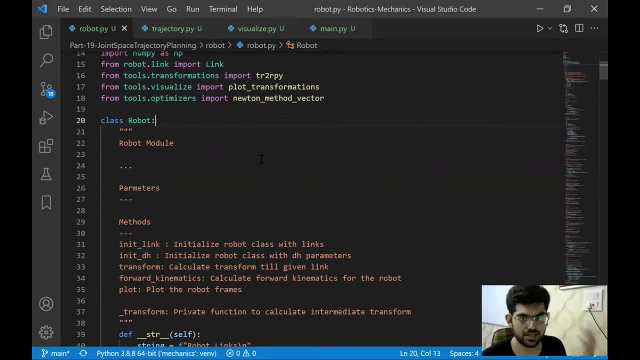 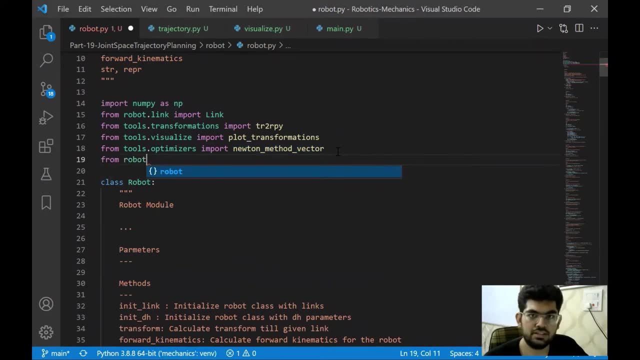 And, finally, we are going to use all the concepts that we coded earlier. So let's get to this. OK, so the first thing that we need to do is import the different trajectory planning algorithms that we are going to use. For that we are going to import The first one is the cubic trajectory planning. 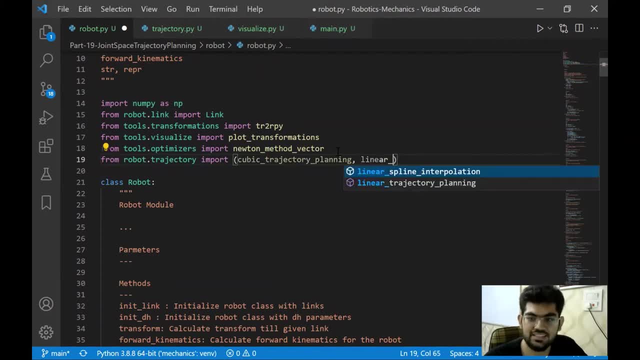 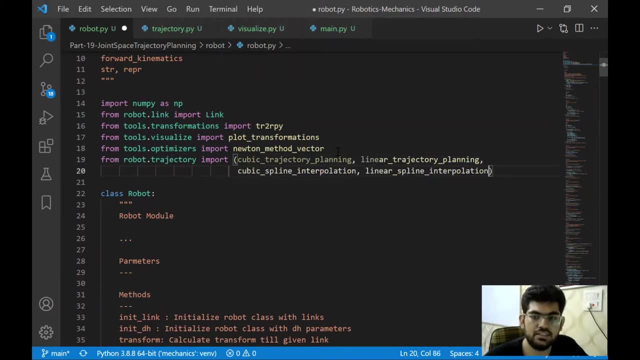 And then we have the linear linear trajectory planning. Then we're going to pull the cubic spline trajectory and the linear spline trajectory. So these are the four main trajectory planning that we are going to use. We are not going to use quintic trajectory as of now, but these are the four that we are going to use. 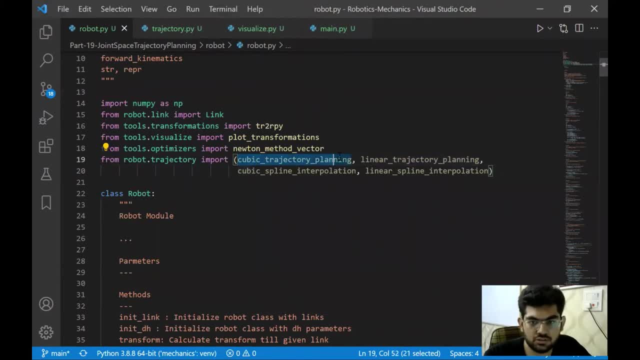 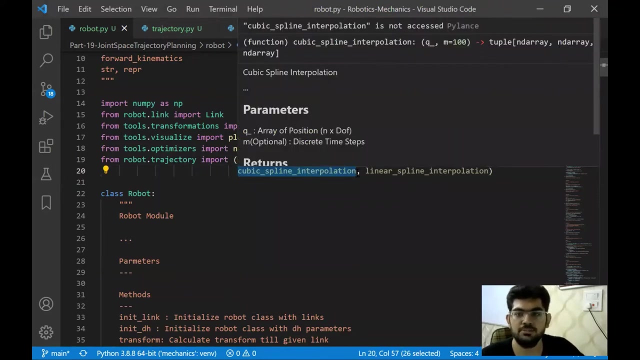 Now, why these four Cubic trajectory planning? We are going to use this if the user passes two points, like the initial point and the final point, But if the user also passes more than two points, like the via points, and as such, we are then going to make use of cubic spline interpolation. 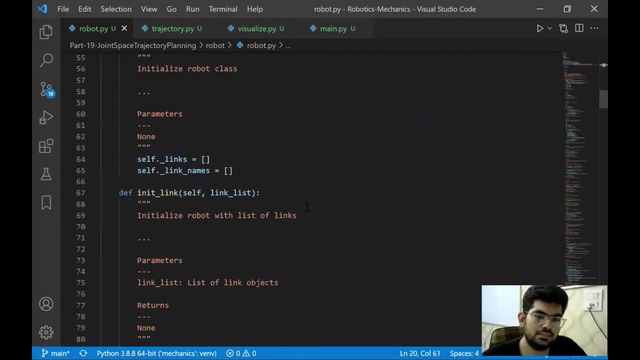 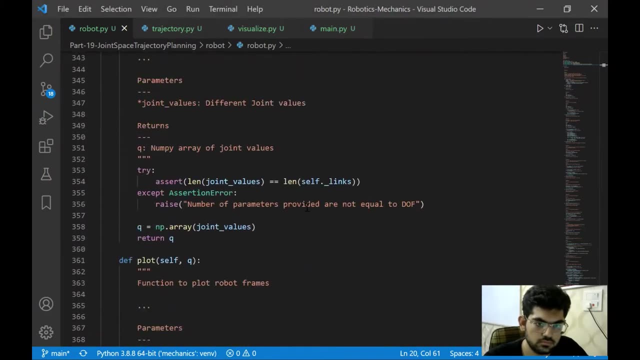 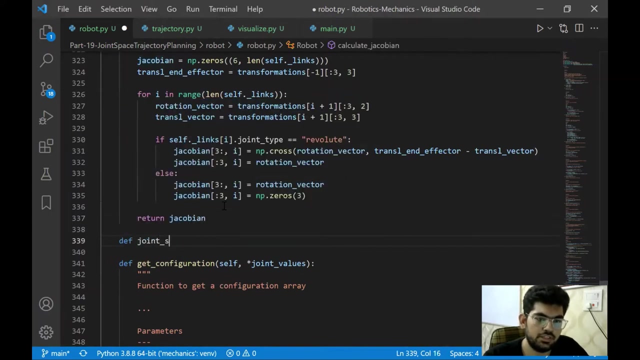 All right, So we have imported these modules. Now let's get to writing the function for this. So we're going to write the function over here before get configuration and we're going to name it joint space trajectory Now as input. the first input is going to be positions. 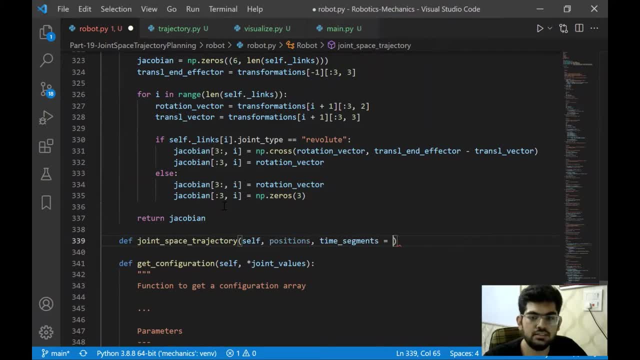 The second input is going to be time segments. This is this. time segments will only be used when the user opts to use the linear trajectory. Otherwise, if the user opts to use cubic trajectory, then time segments will not be used. This variable will not be used, And then we can specify the interpolation that the user wants. 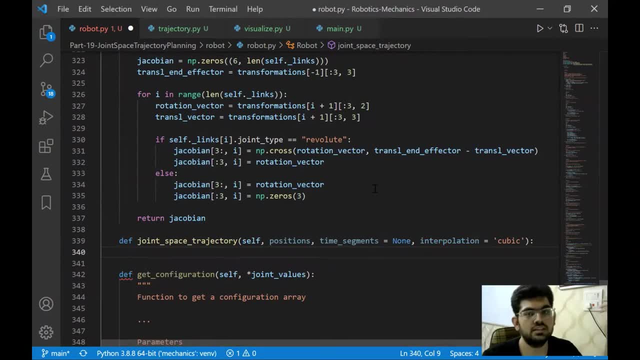 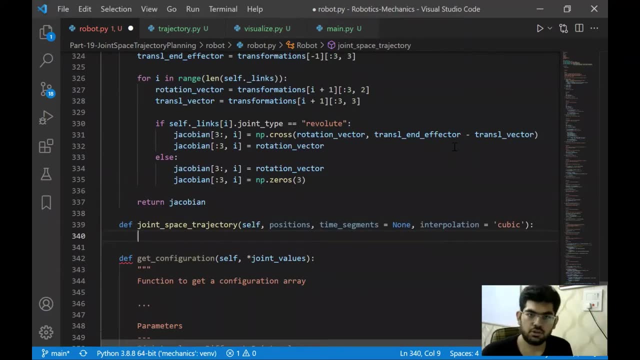 The default implement interpolation is going to be cubic, but the user can specify it to be linear as well. All right, As time goes by, if this project develops, when this project develops, we are going to have more than this cubic and linear interpolation. for sure. 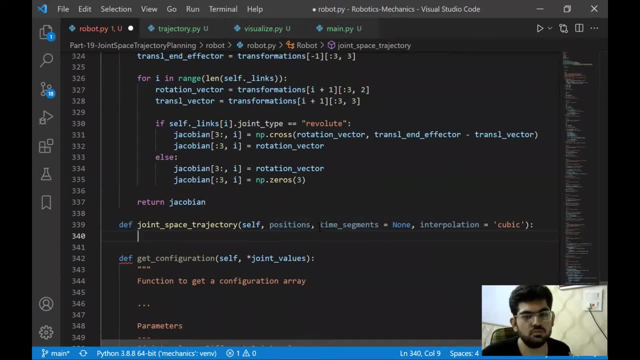 In that case, this function would not would need to be modified as well to take care of this time segments. When we introduce new interpolations, new kind of parameters will evolve over time. Then we need a more general method in order to deal with the different interpolations. 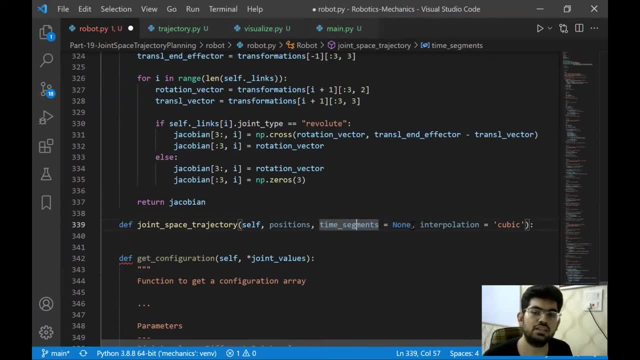 Currently there are only two types. Therefore we can work with that time segments variable, But when the usage increases or the interpolation, the number of interpolations increase. we need to fix a general kind of structure for this. But right now we are OK with this. OK, so now let's add some documentation. 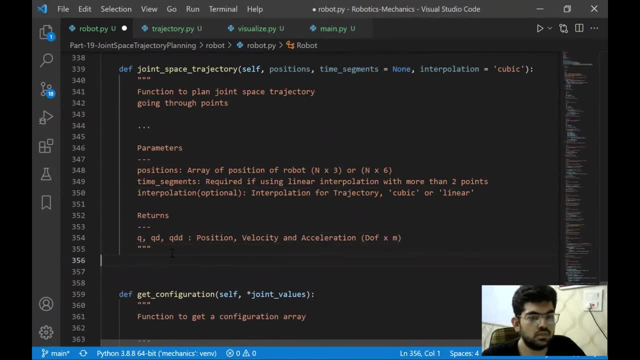 OK, so here we have it. now. In this joint space trajectory, the user is going to pass in the positions. Now the size of these positions can be changed. They can either be n cross three or n cross six. The three represents the XYZ and six represents the XYZ, along with the roll pitch yaw. 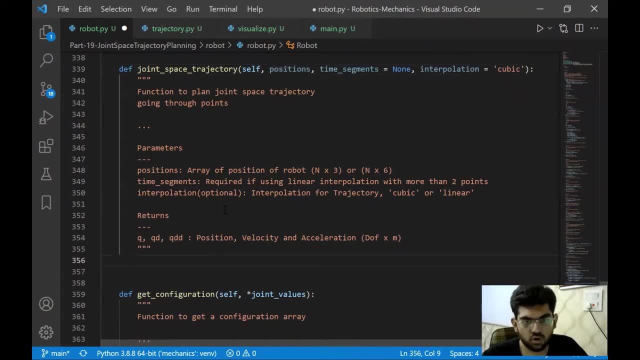 So those are the two that we require. Moreover, since joint space trajectory is more of a user function than a developer function, we are going to need assertions over here, So let's add them as well. So the first assertion is going to be: we're going to assert: if the positions dot shape zero. 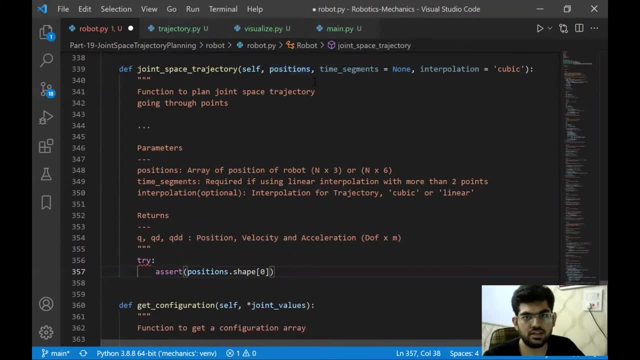 Now the positions dot shape has two components: a zeroth component and the first component. Now the size that we are requiring is n cross three, And we require that the n size is greater than one. Only one point can be planned, So we require at least two points for the planning to make sense. 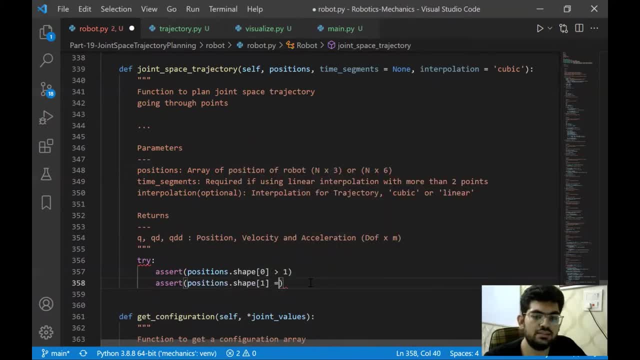 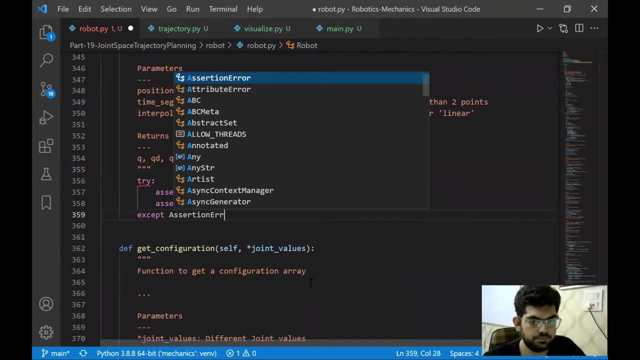 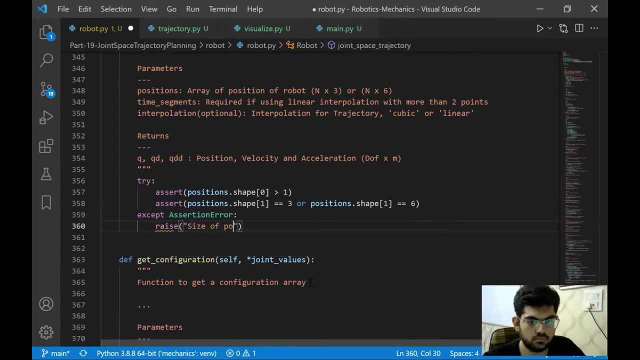 And the second assertion that we're going to make is that the shape should either be equal to three or equal to six, as we have defined, And we can have an assertion error in case this is not accepted. All right. One more assertion that we require over here is for the interpolation. 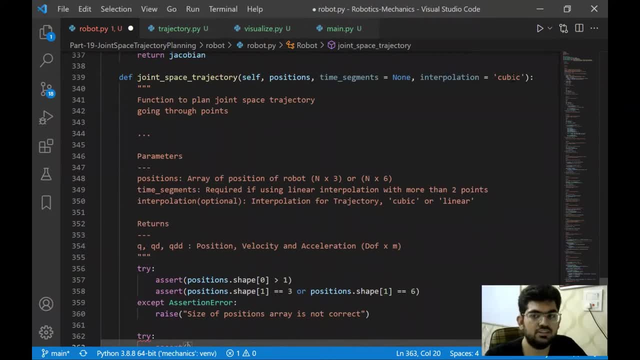 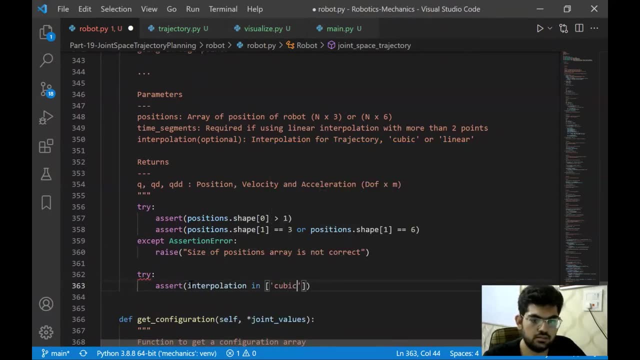 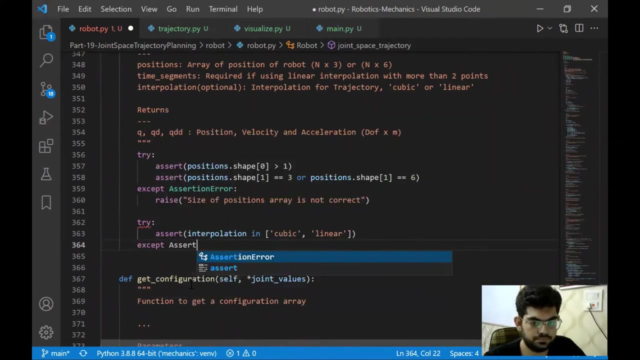 The user. if the user by mistake enters some other keyword other than cubic or linear, then we should also return an error. So let's do that, And we have interpolation in, So it's not. if it's neither one of these, then we are going to raise an error. 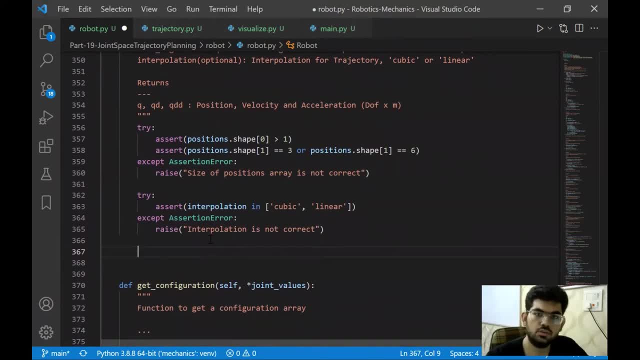 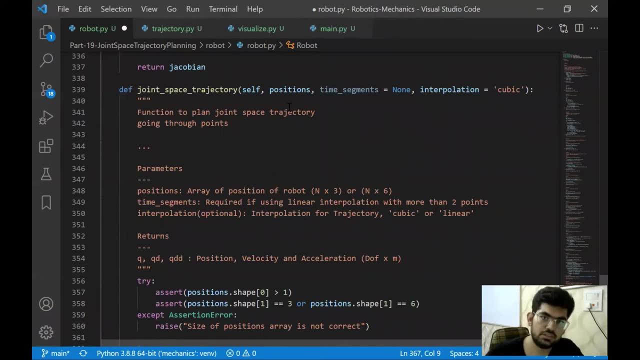 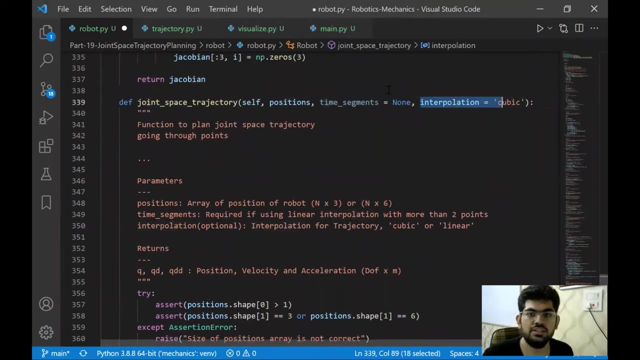 All right. Now the first step, the overall procedure of this whole function, is going to be something like: we are going to take these positions and convert these to joint Values. Then we are going to have an if else kind of statement where we are going to select based on the interpolation and the size of the positions at it. 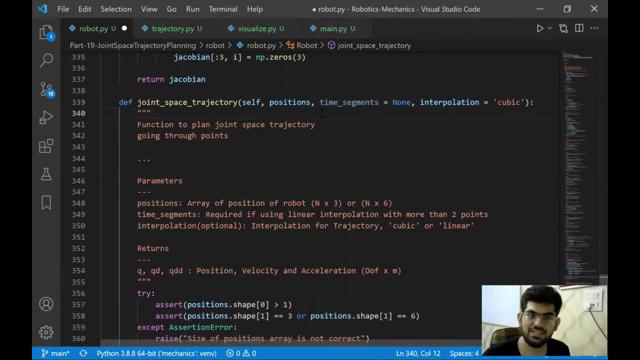 Whether we are going to use this line, the linear spline, the linear trajectory, cubic spline or cubic trajectory. So once we have decoded all those things using a file, then we're going to calculate the position, acceleration and velocity And then we are simply going to return this. 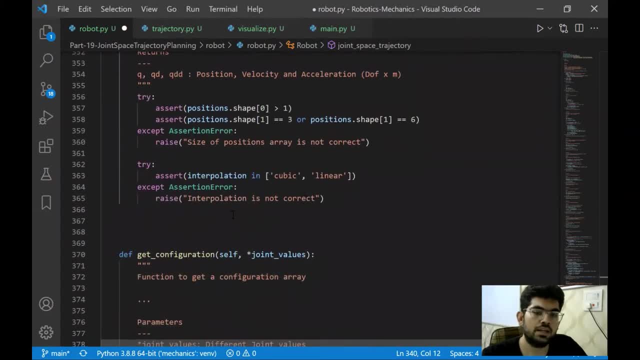 So this is going to be the overall flow Of this function, Right? So the first step that we need to have is convert the joint values. So let's add a comment related to that as well. Now we are going to make use of the functions that we have developed previously to convert the position to joint values. 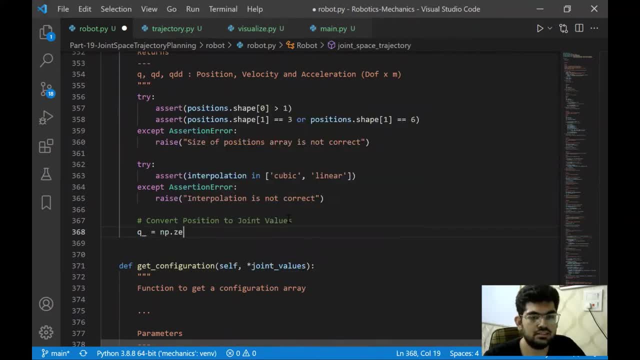 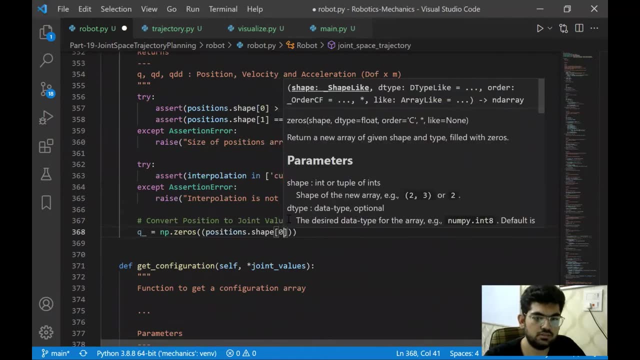 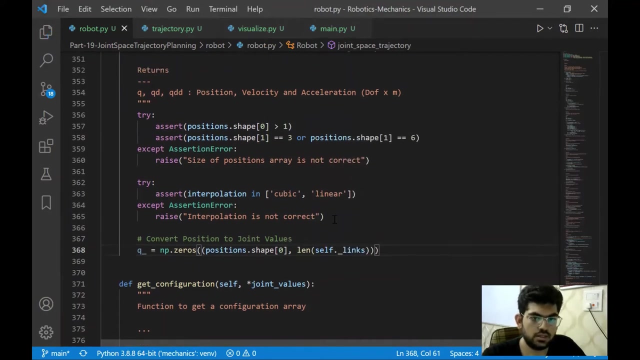 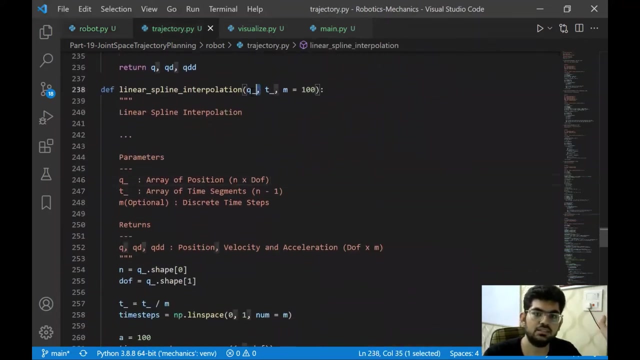 So, first of all, we're going to initialize a joint value- zeros at it. Now, the size of this is going to be positions, Dot, shape, zero, And let's just go ahead and then I'll explain what this means. OK, so that was the. this joint array is going to be a shape similar to what we have described in these functions. 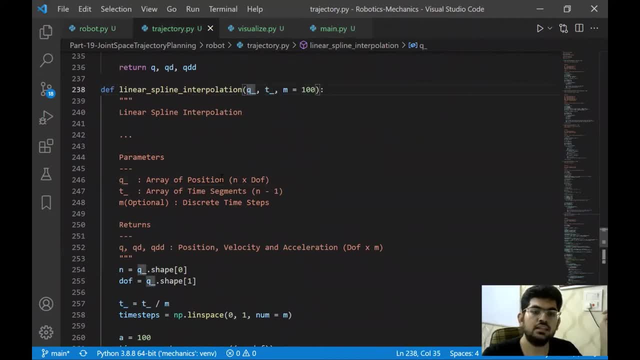 You underscore over here in the trajectories We have already described. the input should be of the size and cross degree of freedom and is the number of points and degree of freedom in the degree of freedom of the robot. We need to have a similar Kind of shape when we are going to input this. 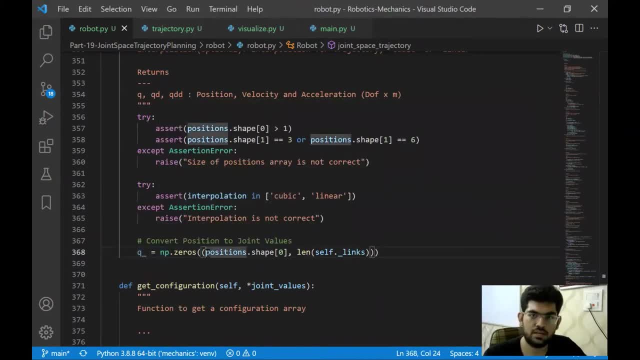 So that's why we're going to define a QQ, underscores and zeroes matrix, that is, of the shape and the number of points and the degree of freedom of the robot. All right, Now the function that we have already made for the robot, The forward kinematics function. we are going to use that, to make use of that. 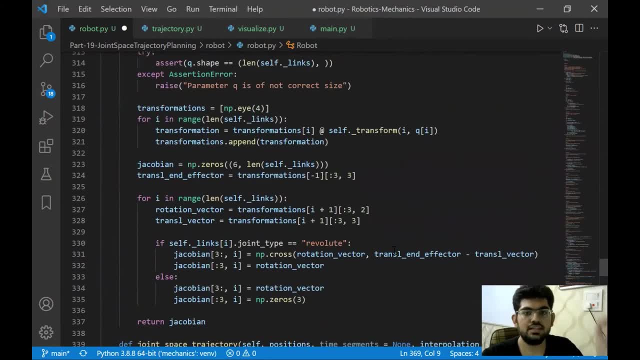 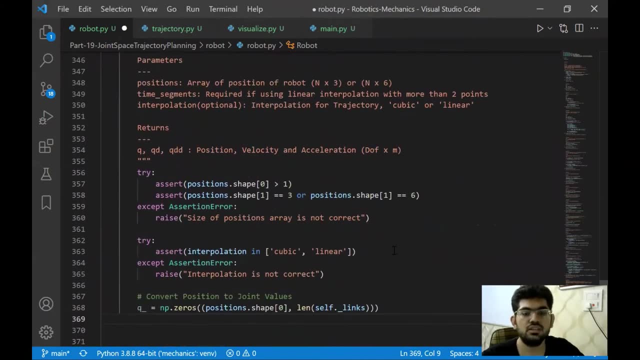 But the one simple thing that we need to see is that the function that we have defined before. They work only for a single position and a single orientation. They do not work as such for multiple points that are passed together. We should have implemented that. 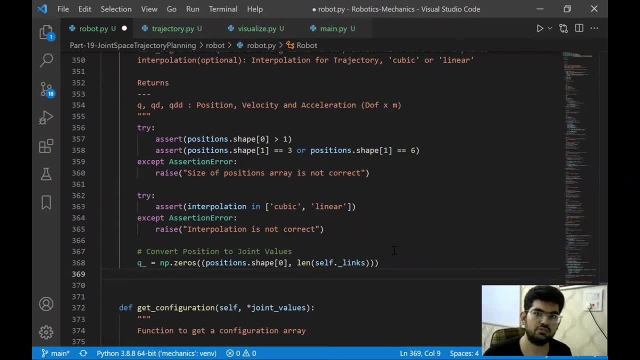 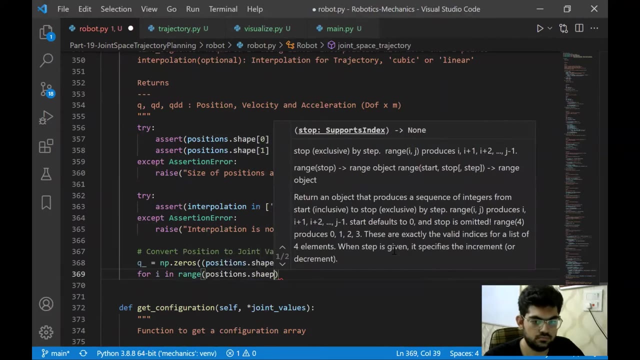 But since we this is our first iteration of the software that we're working on, we are simply going to have a for loop over here That's going to keep iteratingly convert all the position to joint values. So let's do that, for I in range. 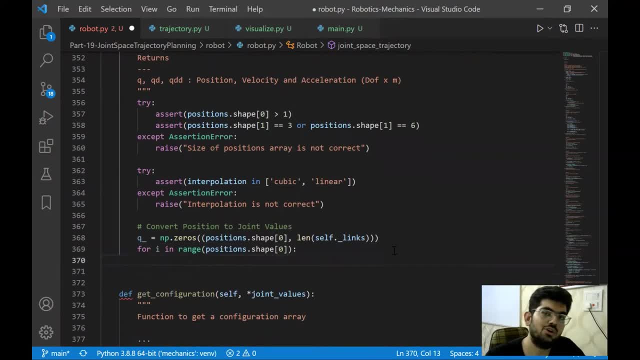 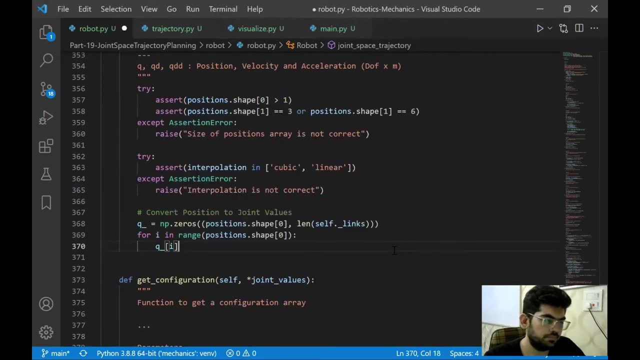 So we're going to loop over the number of points, all the points, and convert their project joint values. Right, This is how we are doing it. We are given the position in space, the X, Y, Z, or we could also have been given the RPY. 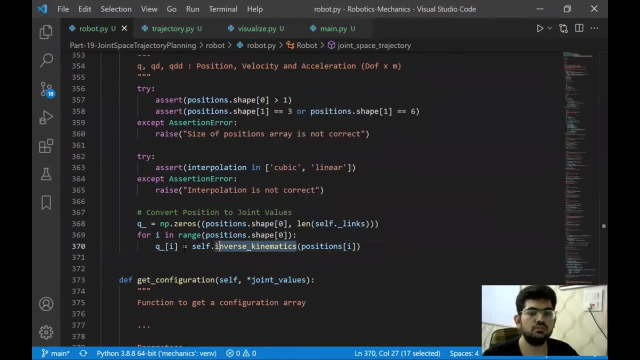 We are using the inverse kinematics function to convert That back to joint values. So right Now, the next step is to add if-else statements, or we can simply say we need to calculate the trajectory from now on. So let's add those first. 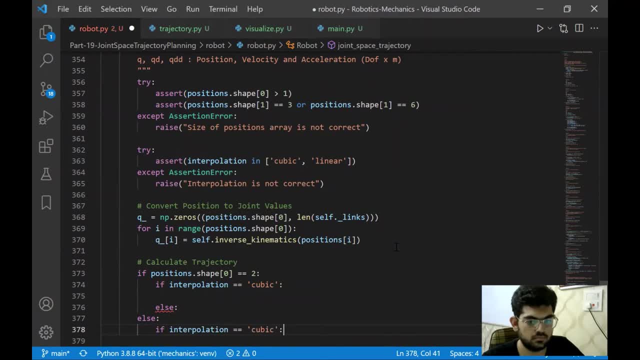 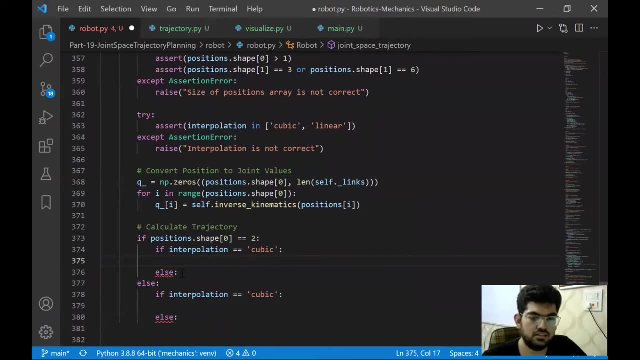 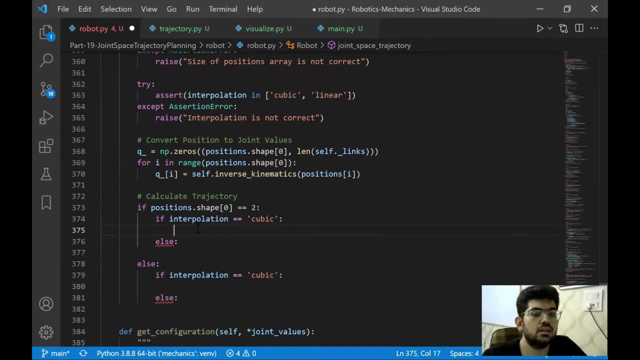 So these are all the if-else branches that we're going to have this over here as well. So there are going to be four cases all in all, as we discussed. One thing important that we need to notice over here is that this is a very- I would say a very- narrow kind of approach to towards this as the code develops. 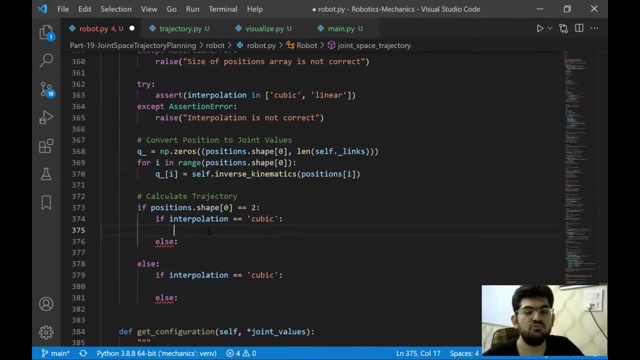 As we have more interpolation methods, we would need to work on a more general method of calling these. Simply increasing the if-else statements would not be kind of acceptable, because this would make the code more jumbled up and all. So that's something that we need to consider in the future when we are going to be developing more on this project. 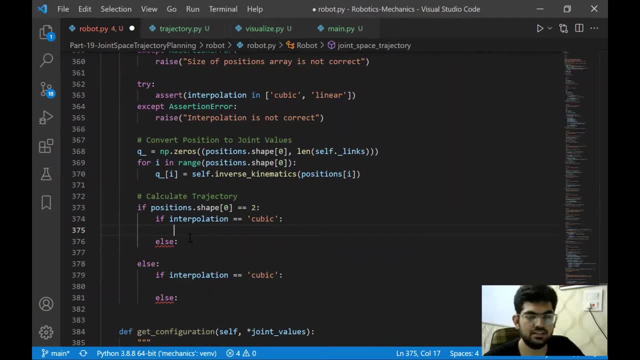 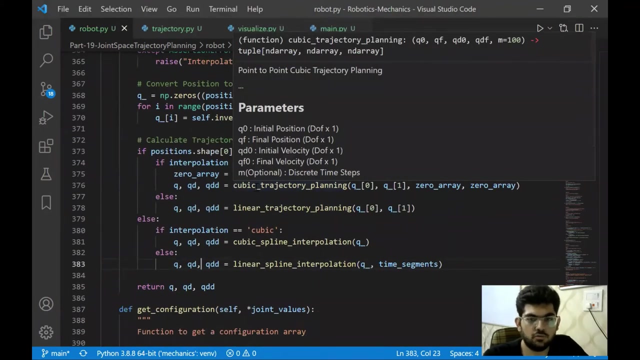 All right, Now we have the four cases and let's input all the variables and get the output. Then we are going to return the position, acceleration and velocity, So let's do that, Okay, So this is the overall structure For all these trajectory planning. we are assuming that the initial and final velocities are going to be zero. 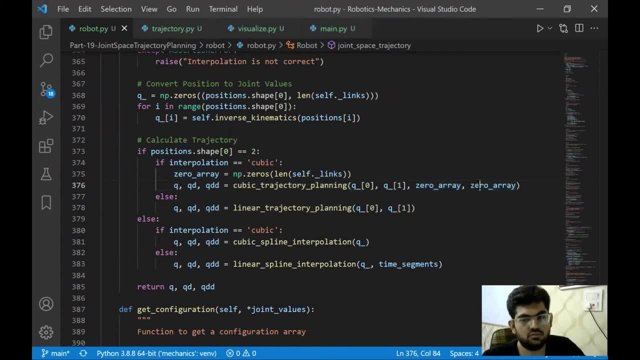 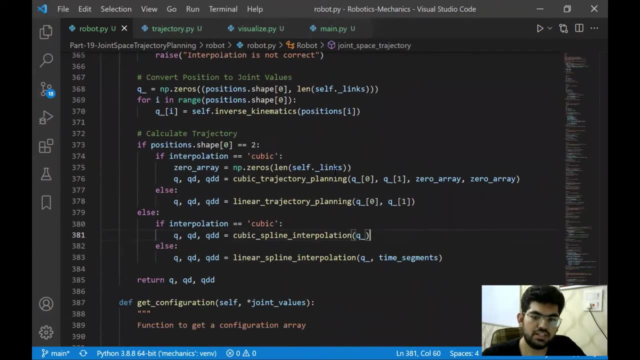 That's why we have passed the zero array over here. Rest of all the algorithms already generalize the case that we are passing in the zero velocity. One thing more that we need to take care of is adding a time assertion for this linear time segments as well. 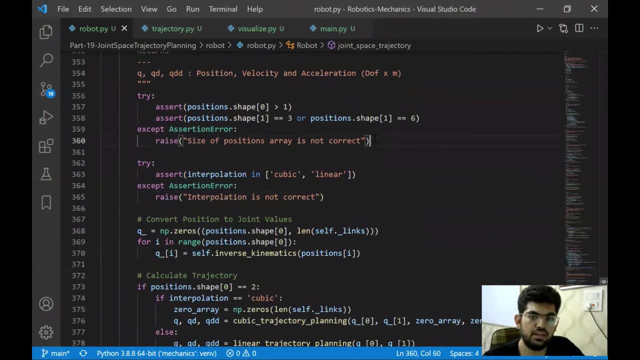 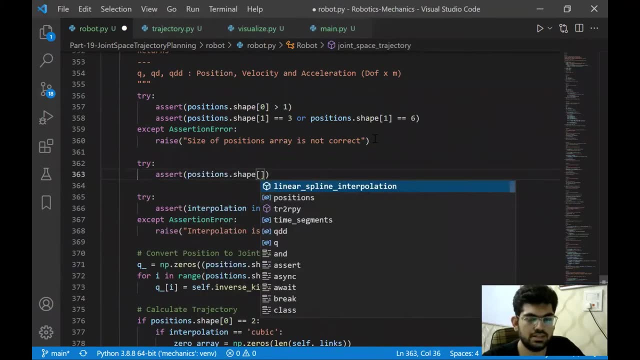 So let's do that. I think we can add it over here. Now. the size of this is going to be number of points minus one. That should be how it is. Yeah, we can do it something like this. Okay, So it should be something like this. 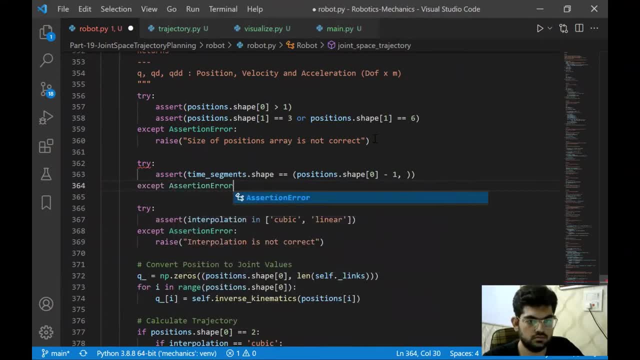 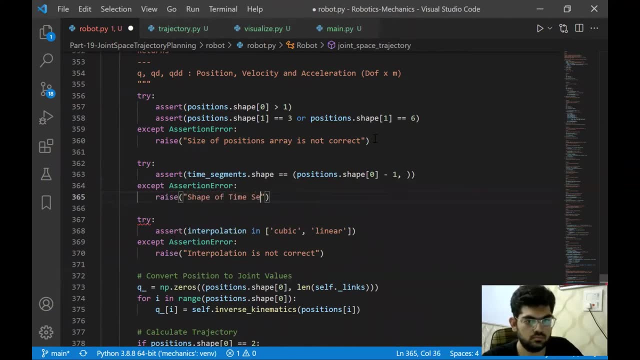 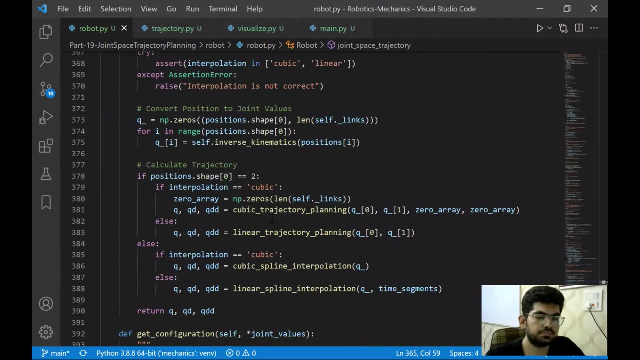 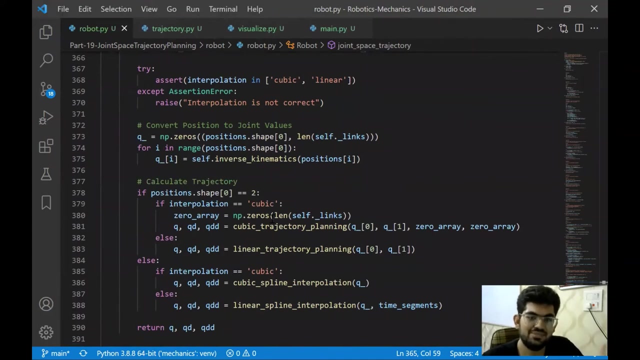 And let's assert: Okay, So here we have this. All right, So now we would be able to generate a trajectory, but that would be all mathematical and variable values as such. Now, in order to introduce some more visual representation of all this, we are going to add a new function to our robot class. 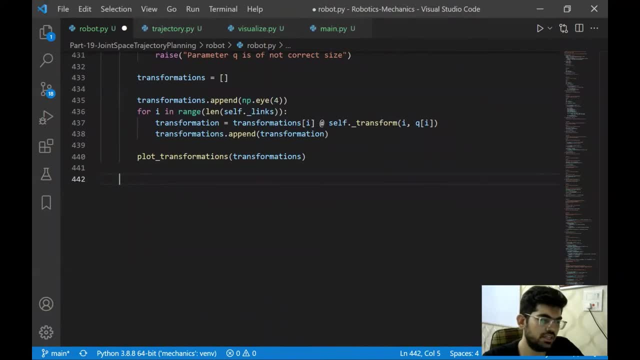 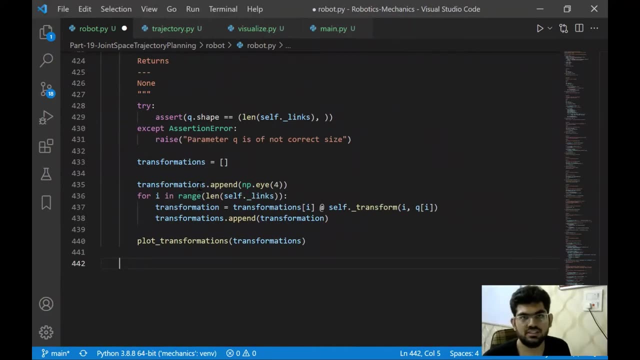 We are going to add that towards the end and that we should be naming as plot trajectory, because this is going to be a function that plots a trajectory for a given robot Right Now. this would require the points that we had developed Self. Q. 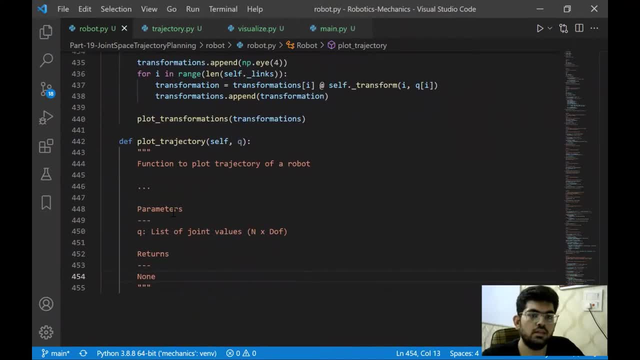 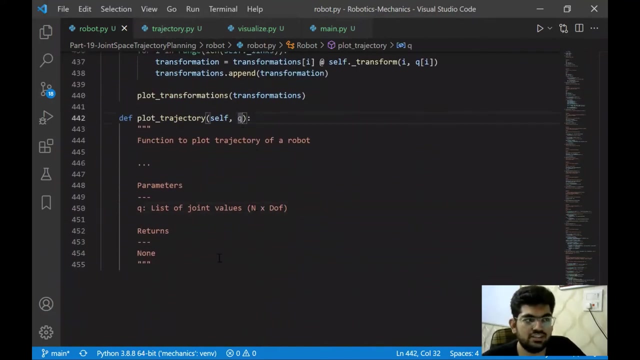 Now let's add some documentation over here. Okay, Now this function takes as the input the variable Q, which is the list of the joint value, The Q that we were returning above in the trajectory part. Now why it only takes Q and not the velocity and acceleration. 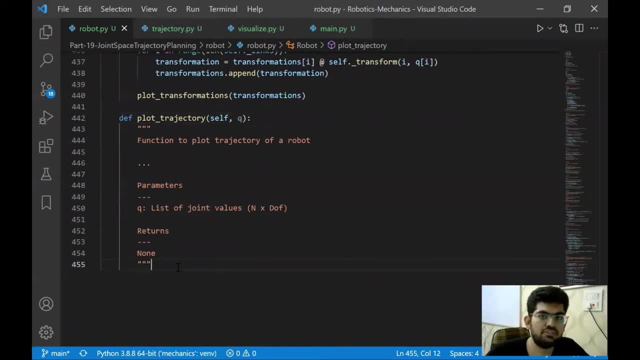 This is going to be covered in the later part Of the videos. In order for the robot to actually move, we need to implement a controller of some kind that is going to follow the trajectory that we have given to it. Right now, we are only assuming that the robot has somehow been able to be, is able to come at the point that we have commanded it to. 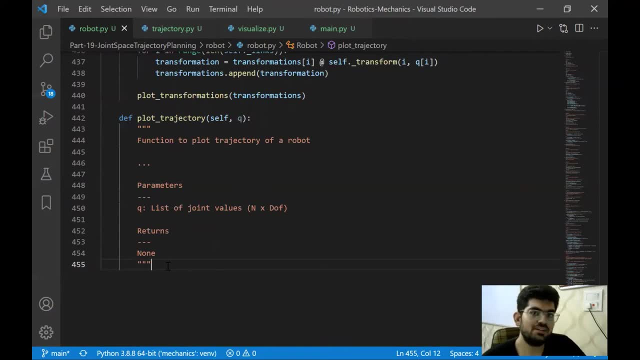 Right now, for the robot to actually come at the position that we command it, We actually need a controller of some kind, which we have not yet implemented, but it is somewhat a plan to implement it in the later videos. Right now, we're just assuming the robot has somehow reached the location that we provided it. 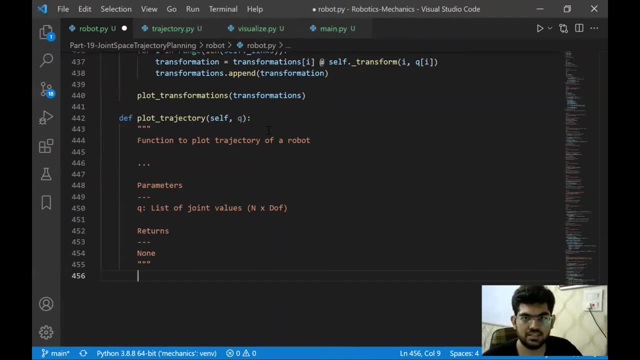 And we are plotting that final thing, that it is over there. Okay, So now, in order for this plot trajectory to work, we need one more new visualized function right in the visualized classes. So right, Let's do that. 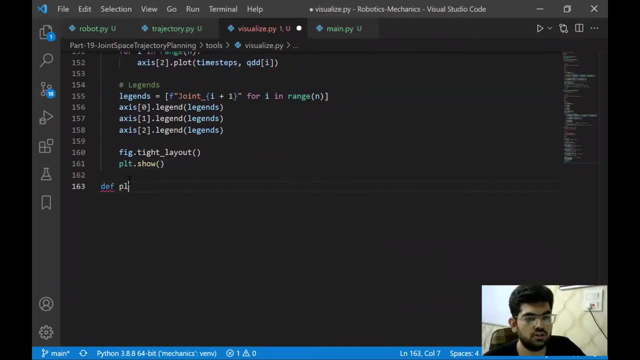 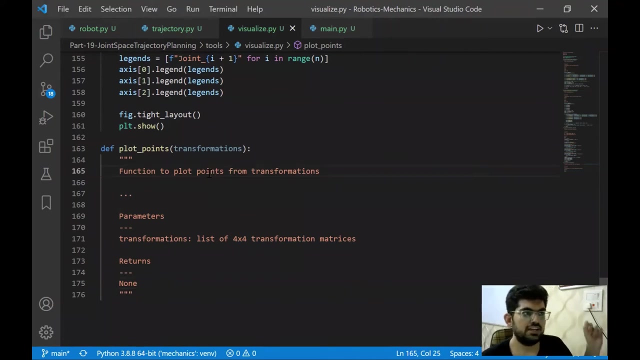 So we are going to define a new function called Lord points, And this is going to take in the transformations again. Right, Let's add some documentation for this. Now, what we are doing with this visualized function is we are going to plot the points that the final end effector is currently on. 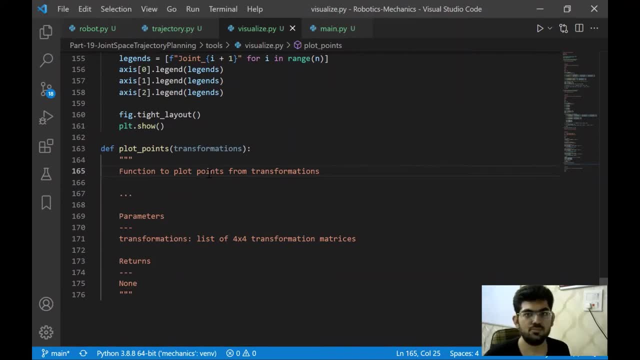 Like for we have, for instance, if we have, a three degree of freedom robot wherever the end effector is pointing the position of the end effector, We are just simply going to plot All those points and see what the final trajectory is looking like for the end effector only. 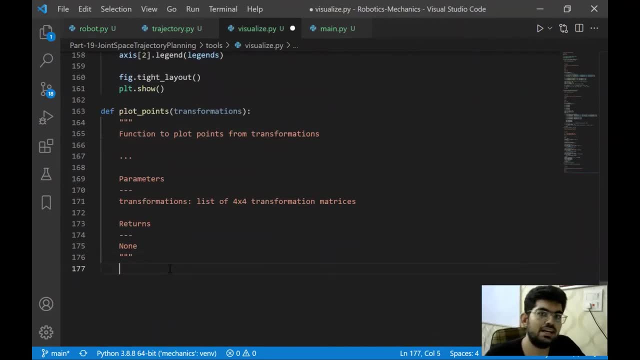 Right For that. we are again going to need a 3D graph and scatter points, like we're going to plot a point in a 3D graph. So that's the overall picture, how it's going to work. Right For that? we're first going to initialize this figure and make it 3D. 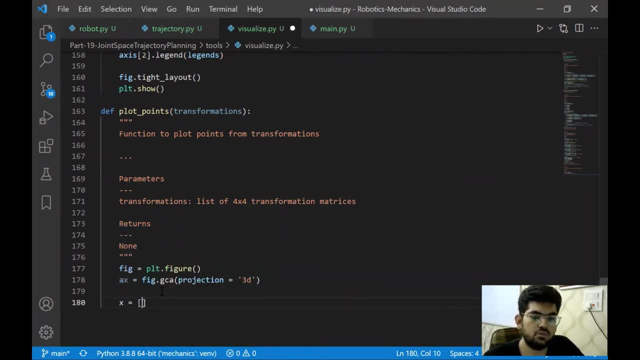 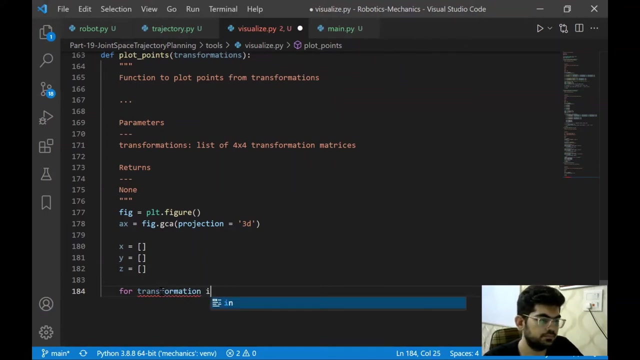 Okay, That's the final thing, Right? So this is done now. Now we need to have X, Y and Z points, And then we're going to look over all the transformations one by one and and append X, Y, Z to the respective lists. 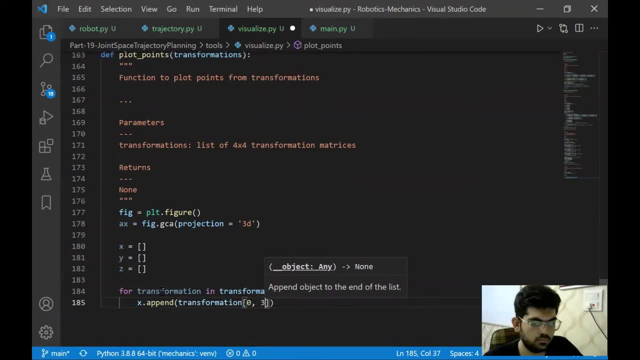 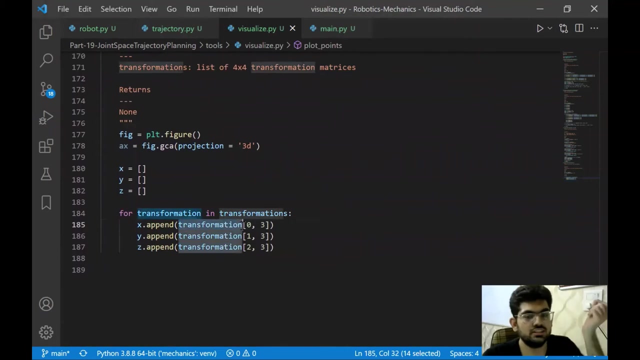 Right, So this is done now. Now we need to have X, Y, Z points. Now, this is very similar to what we have done previously. We are using the homogeneous transformation matrix, and in the homogeneous transformation matrix the x, y, z are located. 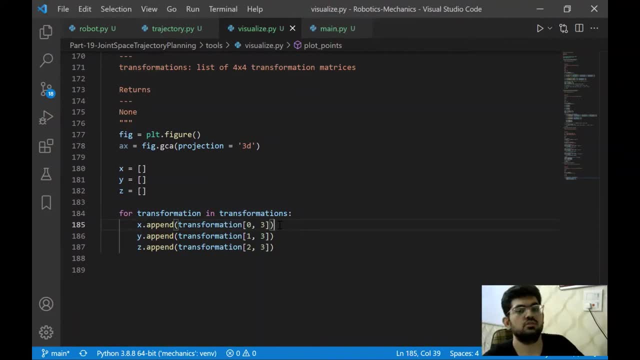 in the last column and the first, second and third rows. So we are selecting those and appending those points to our x y z lists. then we are going to call the scatter 3D function and pass in the x y z that we have and we simply going to then call the PLT dot show. 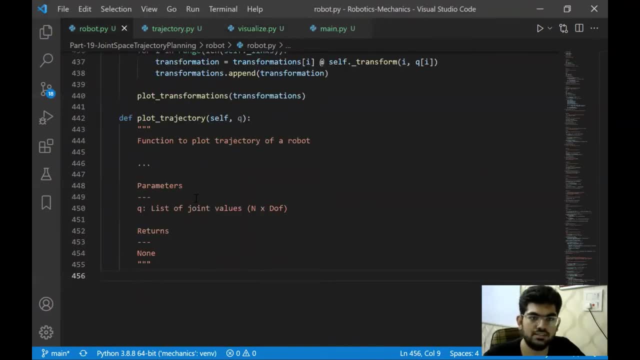 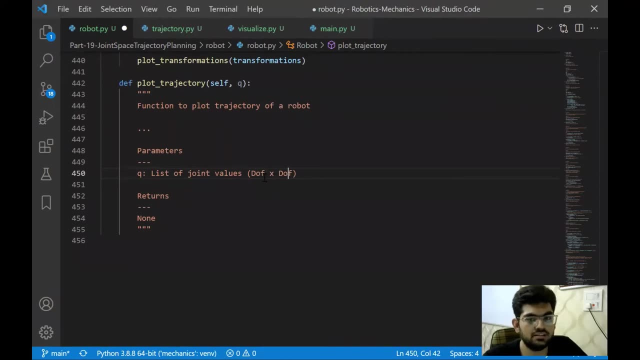 Now, this is the backend function that we have developed. Now we need to add something in this plot trajectory function that we have defined for the robot. So the point, the list of joint values that we are going to add, is going to be of the shape of degree. 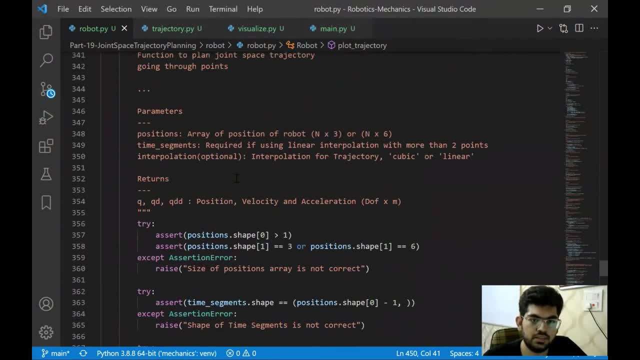 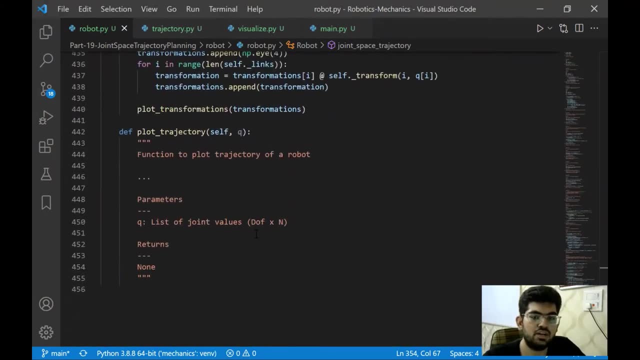 of freedom cross n. as we can see over here that we added, The degree of freedom cross m is returned from all these trajectory planning algorithms that we wrote before. So that is why we are going to have similar structure: degree of freedom cross n. So the first thing, 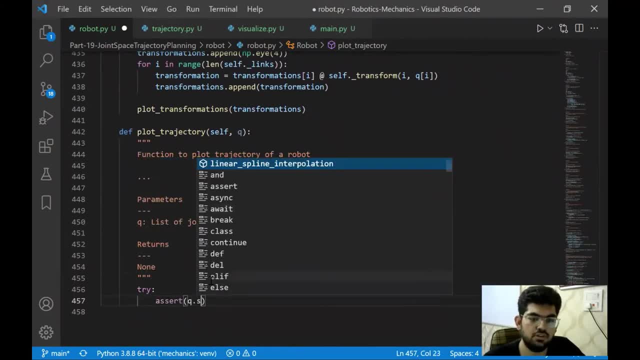 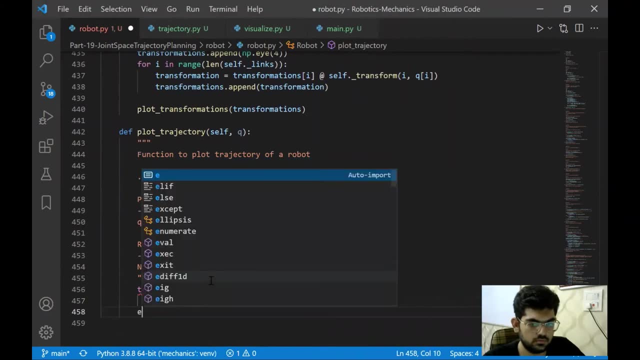 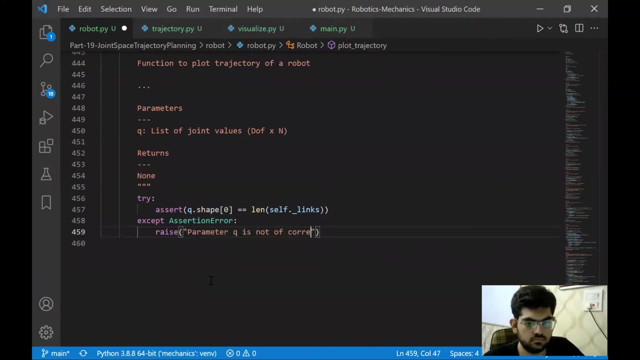 that we are going to do is assert the shape that we have for Q. Now we are going to define. So we are going to define a transformations list and we are going to append all the transformations to it using the forward kinematics function. So let us do that. So this is the final. 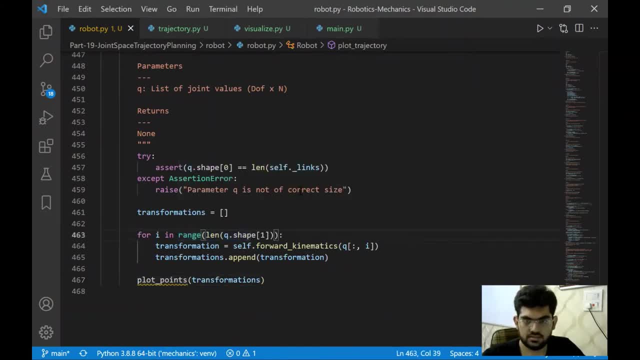 thing that we have. We are looping over the second shape, second index, shape of the Q, and then we are calculating the forward kinematics for all the Q of the, all the degree of freedoms. Right, Yes, we are taking the joint Values at each point that we had just found out using the trajectory planning, and we are 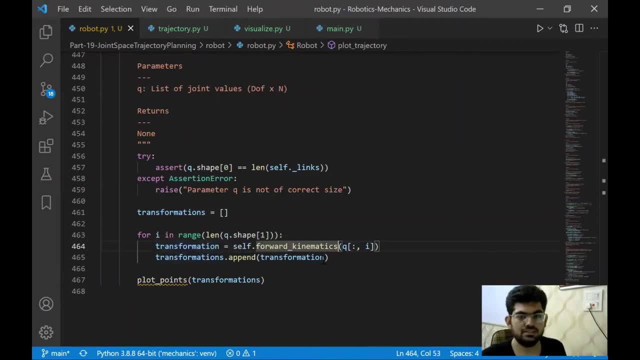 passing it to the forward kinematics function. Then the forward kinematics is calculating the final end effector position: homogeneous matrix. We are appending that to the transformations list that we have and then we are going to call the plot points function. Now this is: 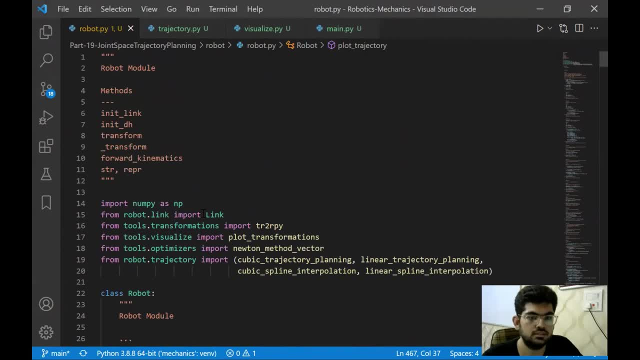 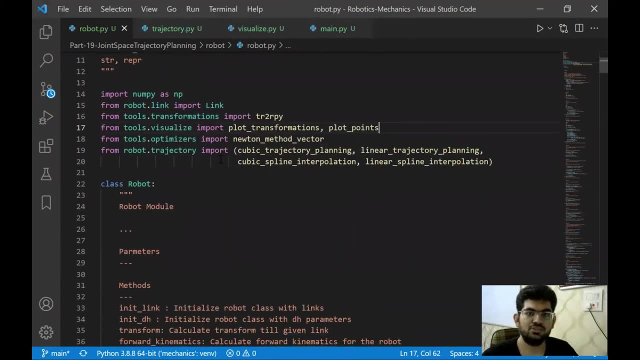 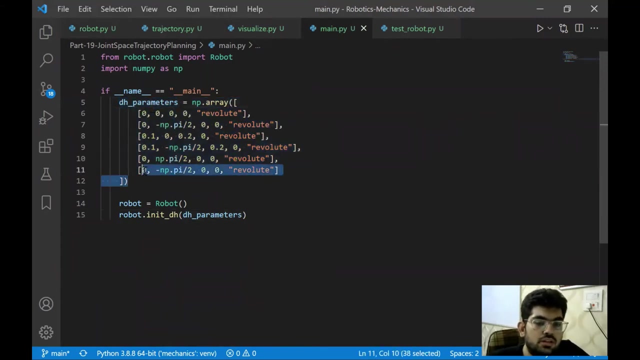 not currently imported. So let us go above and import this. In visualize, we can import plot points, Right? Yes. Now what is left is to test and see how this works. So in this, we have already defined a robot, the Puma robot, the six degree of freedom robot. Using this, we are going to 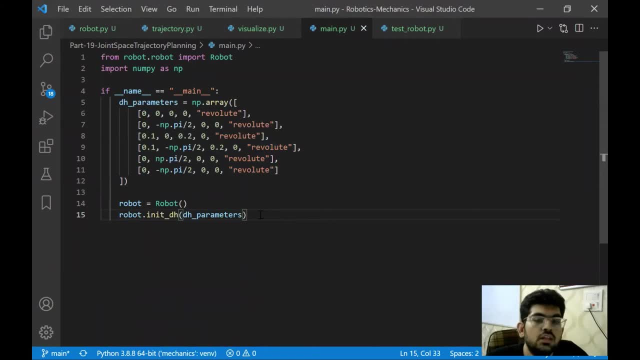 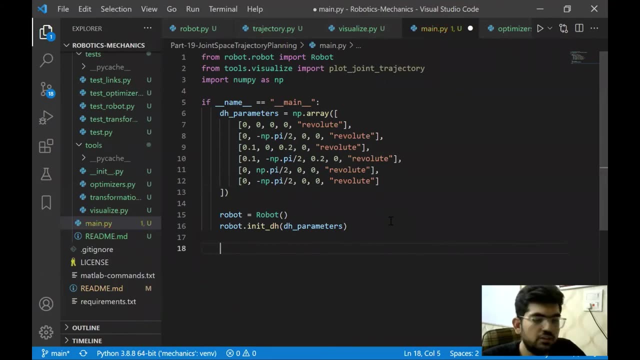 visualize what the different trajectories look like. Now we are going to test it on the mainpy file. How we are going to do it is: first of all we are going to get some configuration from the robot using the dot cut configuration. Now we need six joint values, which are over here, and we are going to create a series of 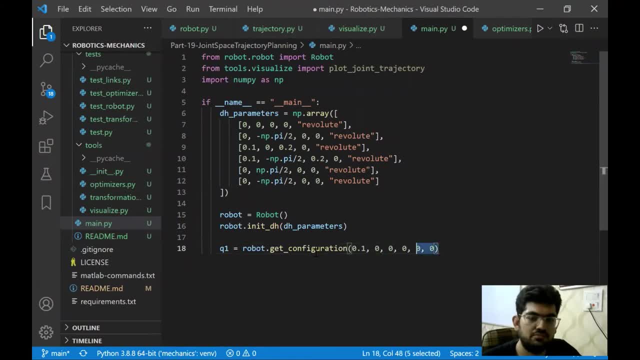 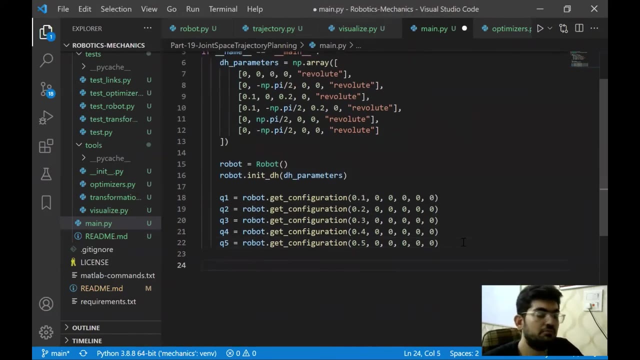 0.1, 0.2 till 0.5.. I think five position parameters. So let us do that first. Okay, Now we have these position parameters, Now let us compute the transformation matrices of these joint values. 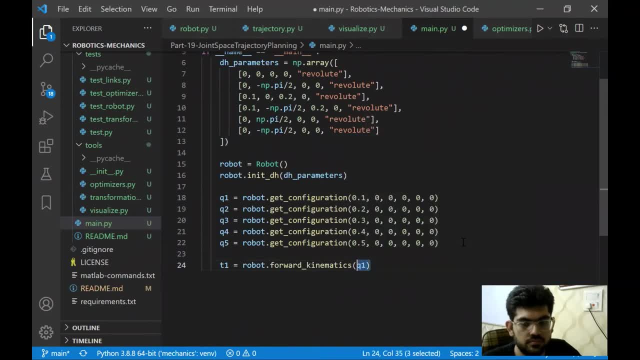 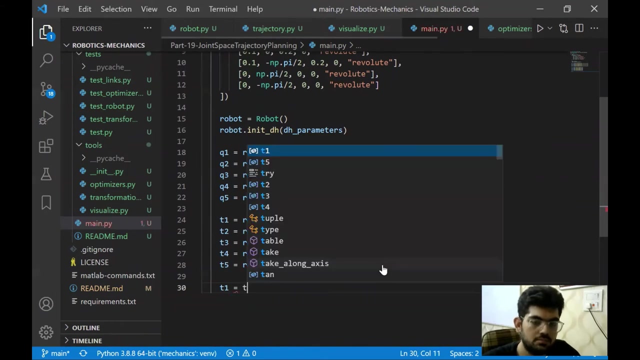 Okay, Now we have these position parameters. Now let us compute the transformation matrices of these joint values. Okay, Now these are computed. Now we are going to subsample them. We are going to get the position sub-area out of these five. 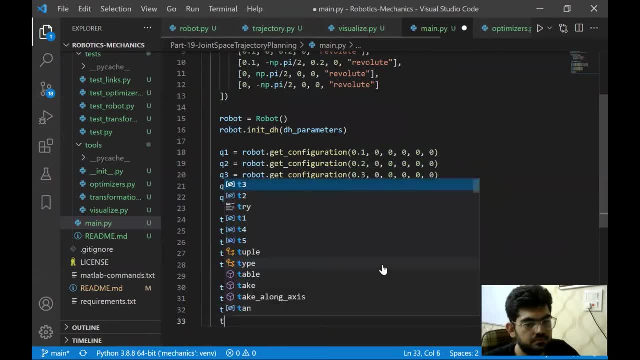 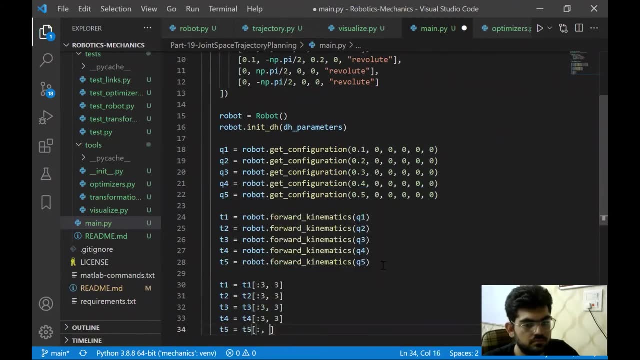 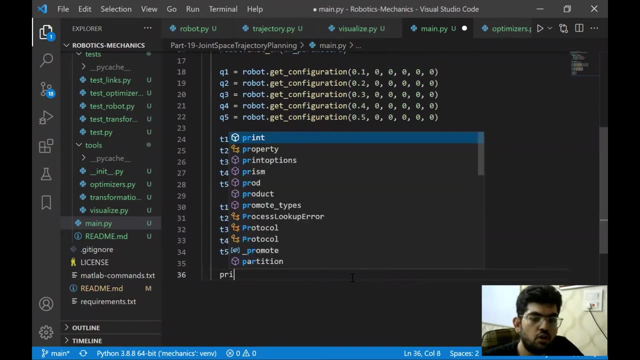 Okay, We are going to add one more: one, two, three, four, five. Okay, So that's it. So we have this now. now, in order to compare the plot that we have, let us print these values as well, Okay. 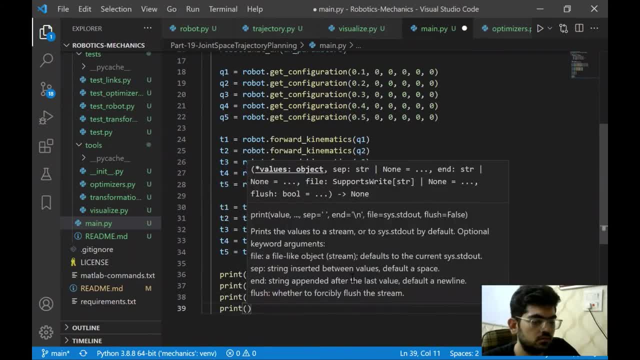 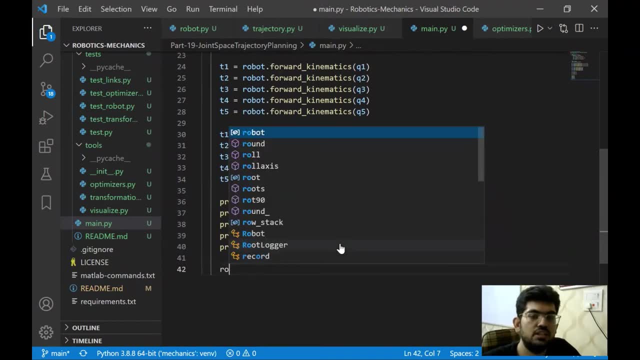 There we go. So you can see that is an supremacy. Now these are printed. now we can get to the joint space planning. First of all, we will create a positions array which is composed of all these values, and then we are going to do some joint space trajectory and we are going to pass in the positions. 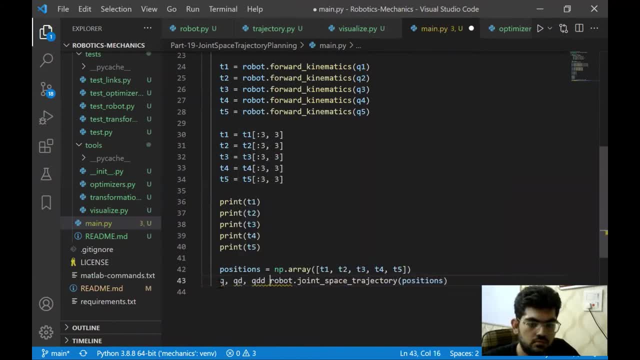 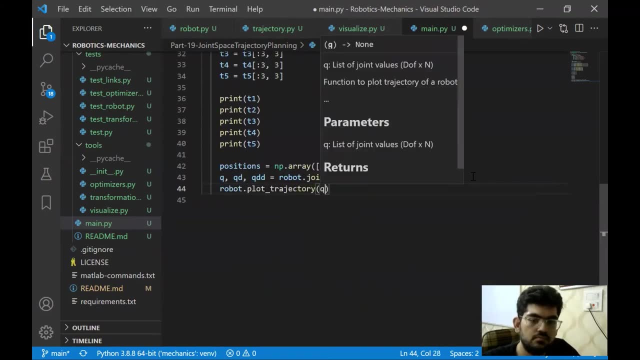 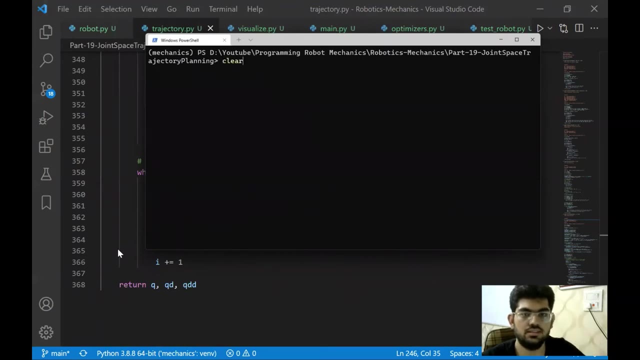 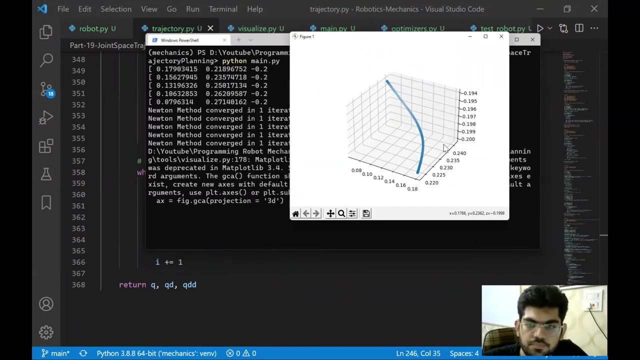 These are passed in. Now we can finally plot the trajectories that we have single trajectory. So now we run this main dot py file. So, as we can see, now we have a value of minus 0.2 for the z, but something does not seem. 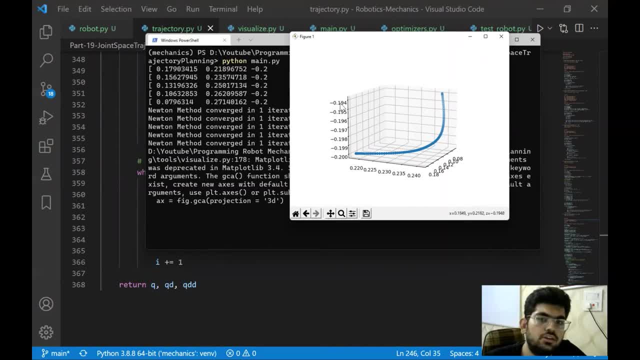 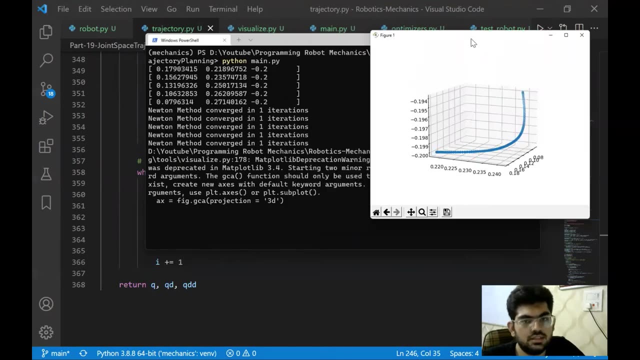 right for this, because minus 0.2 is actually incorrect. So we are going to minus 0.194.. Even if the error was to be allowed, we would have allowed an error of minus 0.199 at most. So something does fail off. and one new thing that we can notice over here is that the Newton 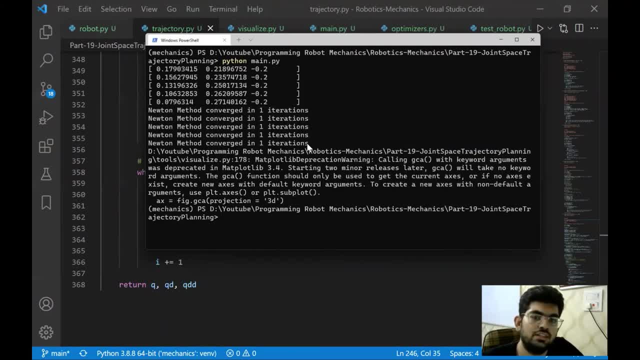 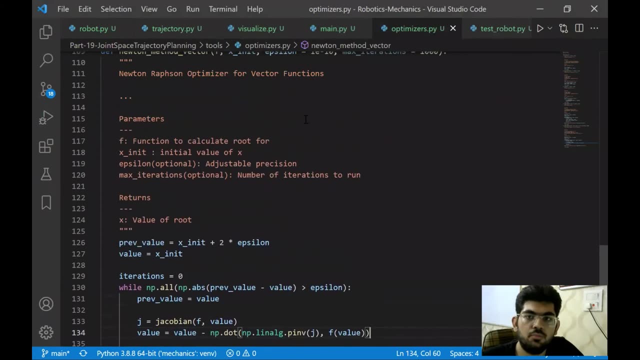 method for all the cases is converging in just one iteration. So there seems to be some problem with the Newton method vector that we have just developed. So let us see if we can find any error. Okay, so in this optimizers file we can see that the NP dot all seems a bit off, because 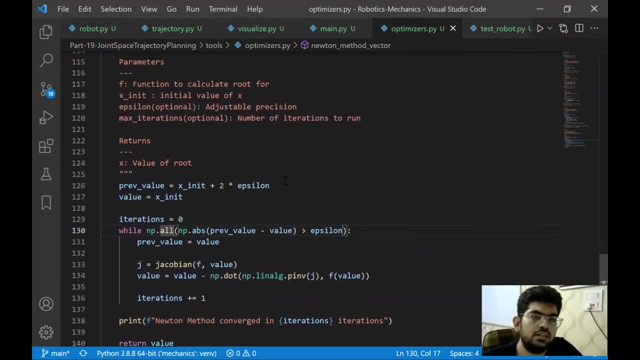 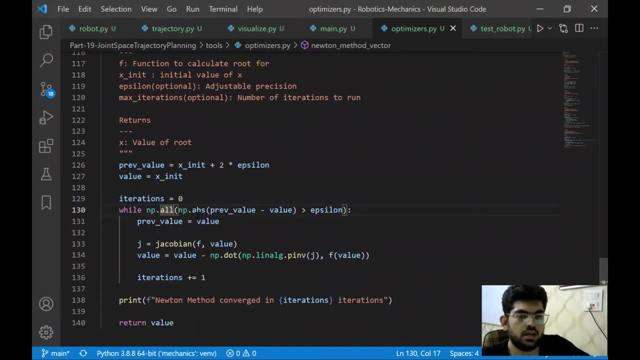 it is terminating the iterations in just one step. So instead of dot all. now the problem is over here. NP: dot all evaluates the things that something like it tests whether all the array elements along a given axis. So in this case it is evaluated to true. 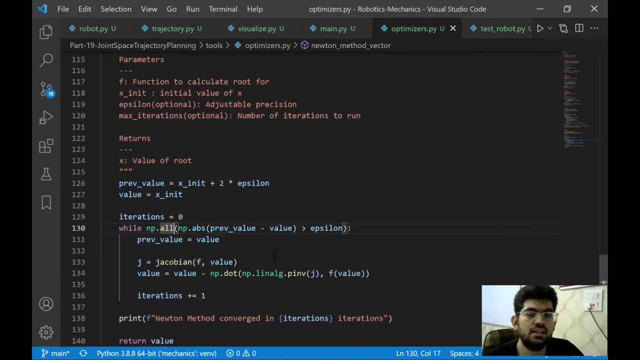 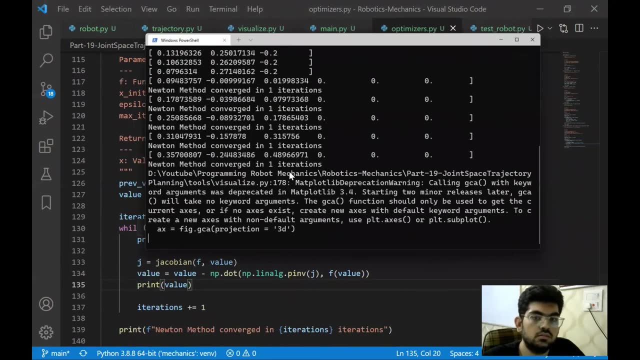 So some values towards the end of the. let us just print the value and see what is going wrong over here. If we just print the values, then we can see the final array points are equal to 0.. Now these are actually going to evaluate to true in our case, because these values are. 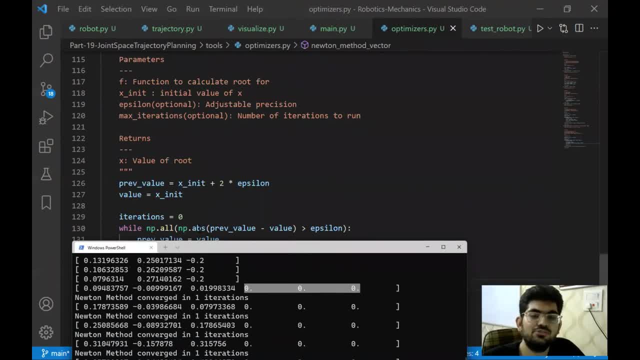 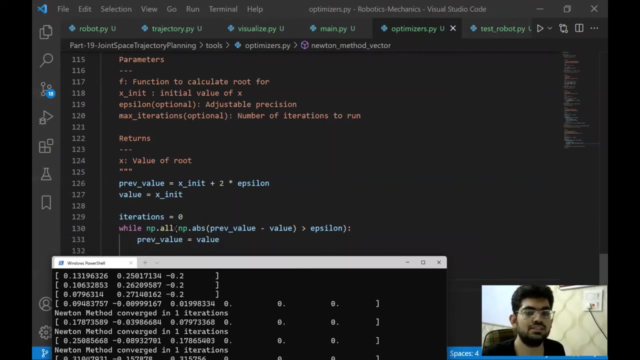 no, these values are going to evaluate to false for this case, For this case, For the pref value minus value greater than epsilon, these values, because of these zero values, our complete loop is going to halt right over there because the NP dot all will. 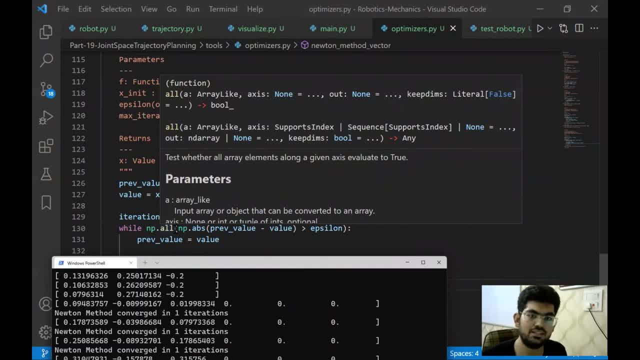 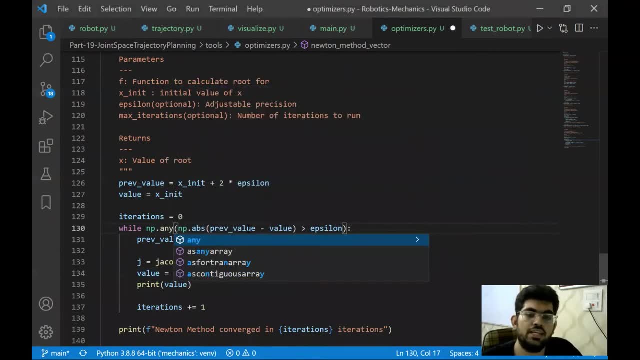 see a single false and it will evaluate the complete vector as false, Therefore terminating the expression. however, what we needed here was NP dot any that would make the while loop go without terminating the expression. Now, this: any checks whether if there are any true values or not. 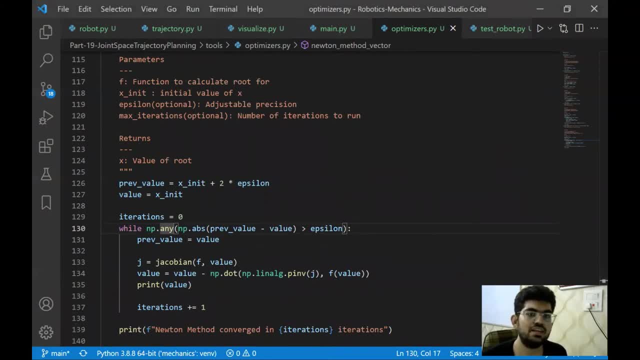 If there are any true values, then it will keep on going the loop. If there exists even a single false value, then the loop will halt And even a single true value right. it will keep on evaluating till all the values that are present in the array are false, and that is what we require for the optimization to 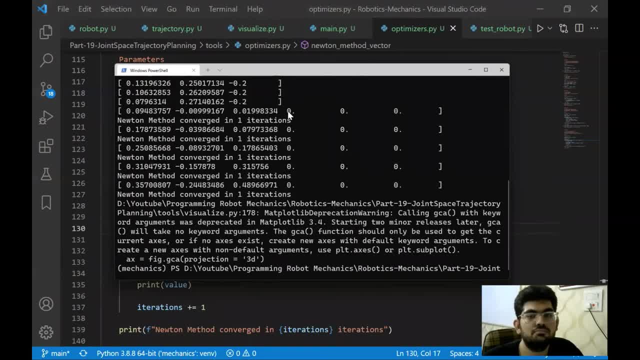 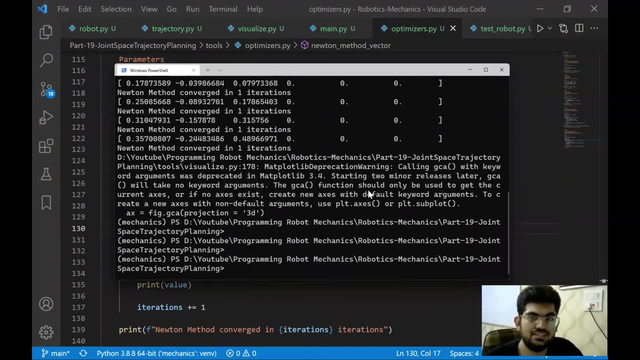 complete. Otherwise, the optimization will be done for some partial vector and not some vectors like these. Now, this is quite intriguing that we were not able to catch this error in the unit tests as such. So, yeah, it's just a learning that we need to keep our unit tests updating like this. 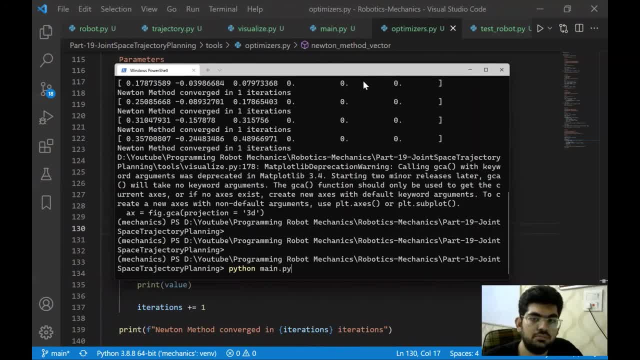 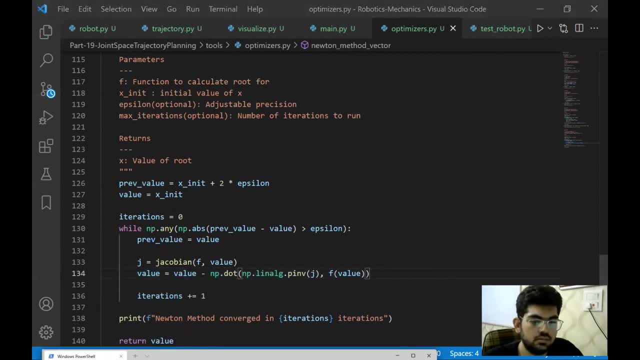 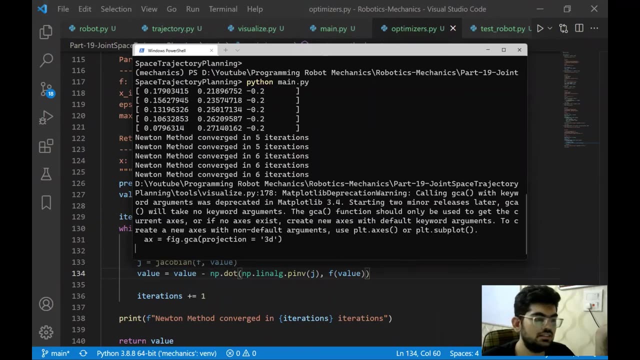 Okay, since we have identified the error and, I think, possibly resolved it as well, now let's run the loop that we have. Okay, let's now run the complete again. Now we can see the iterations have increased: 5,, 5,, 6.. 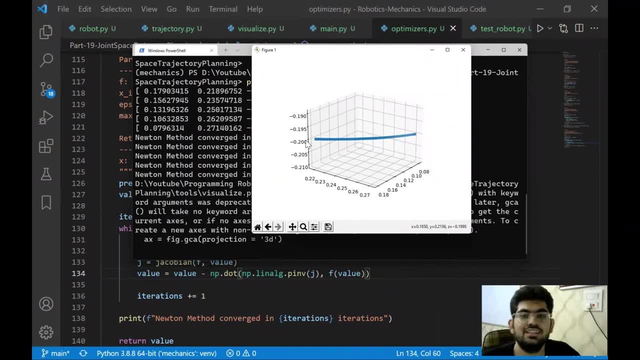 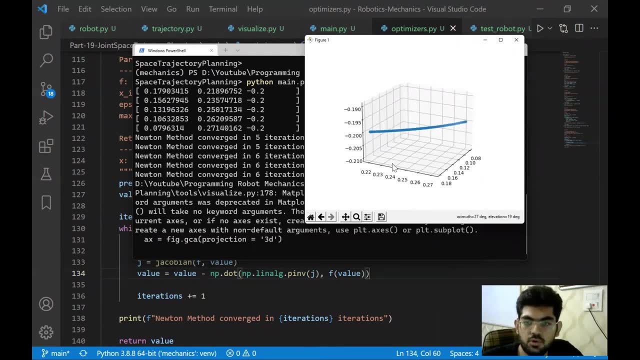 And we can see over here the it now looks really good Like the minus 0.2 is actually traced very well- minus 0.2.- And the 0.22 till 0.27 is also traced very well and we can see the x is also traced pretty. 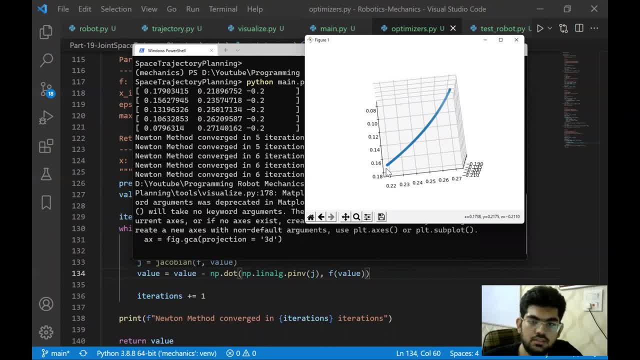 good, Like 0.17 till 0.7.. Okay, Let's run the complete again Now. we can see the iterations have increased 5, 5, 6.. And we can see the iterations have increased 5,, 5, 6.. 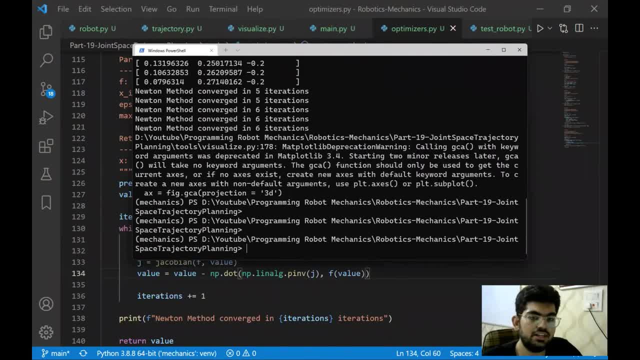 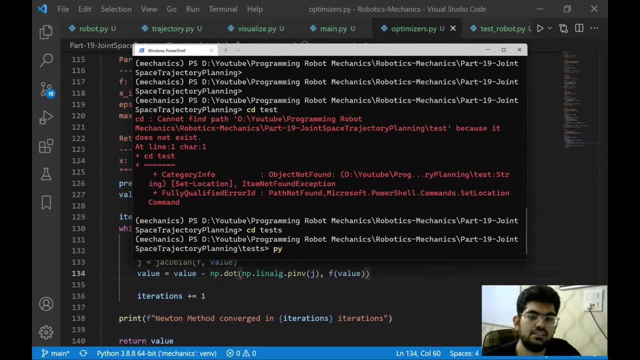 And we can see the iterations have increased by 0.08.. Right, It's looking pretty good. now, Okay, one thing that we need to do, since we have pointed out a new error and we changed some files over here. let's go to tests and run the unit tests again. 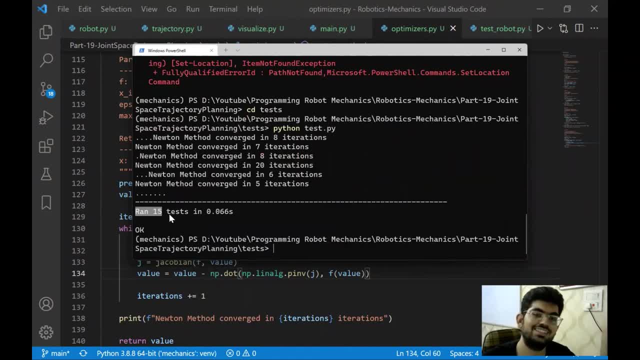 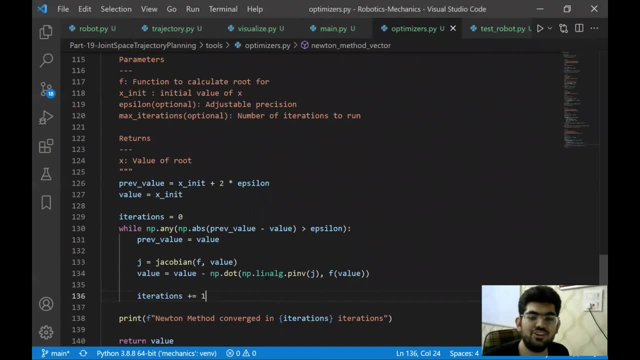 This will ensure that all the things are working fine. Yes, all the things are still working fine. So this is, in one way, we have seen that a unit tests are a little off. They do not check all the values. This is because the unit tests were made for all the values. that 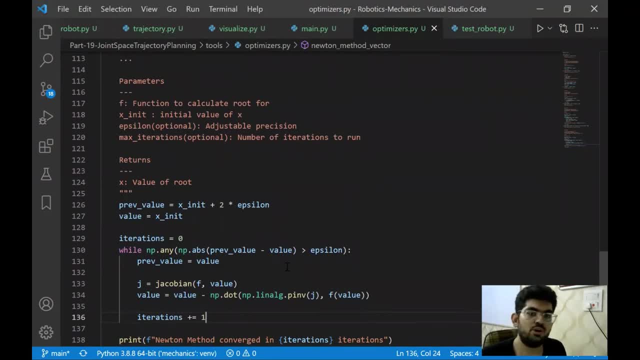 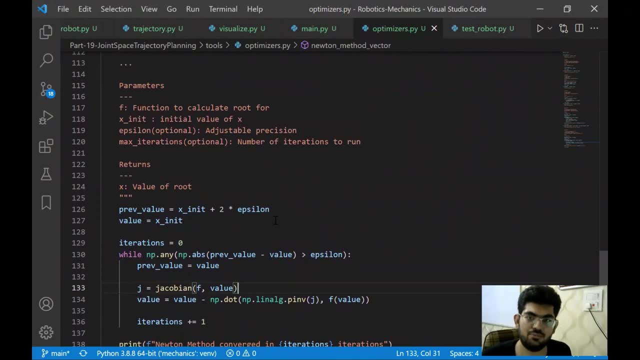 in which there were no all the values needed to be optimized. but in our case, for our robot, there are some values of the joint that are do not require optimization and the loop still wants to run some more iterations over it. that's why we required np dot any over here. 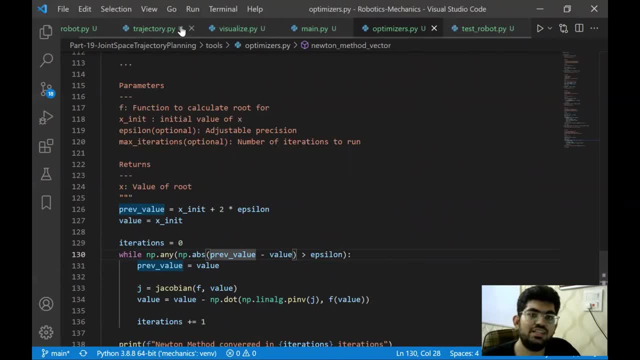 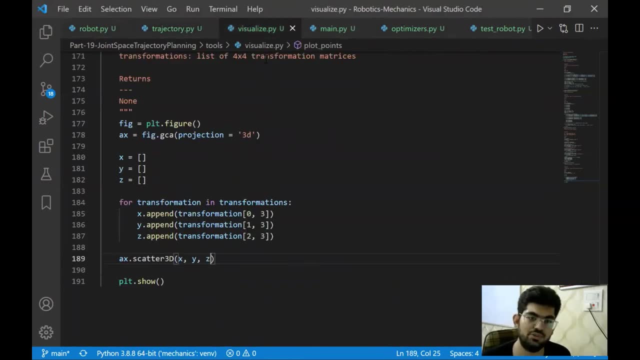 so this is a mistake that we point fixed over here, and this is pretty good, since we are developing the library. this is a normal procedure of developing any software. we need to keep on testing and keep on iterating over our software to compile and exit, compile and fix. 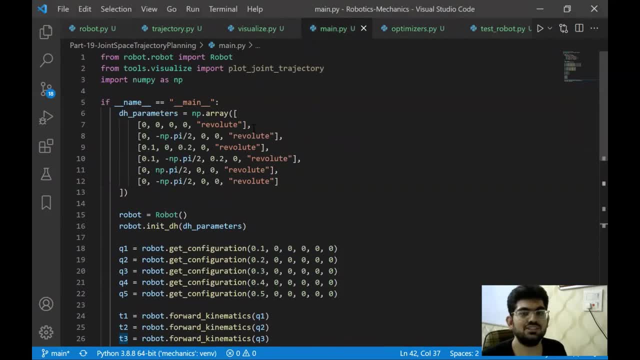 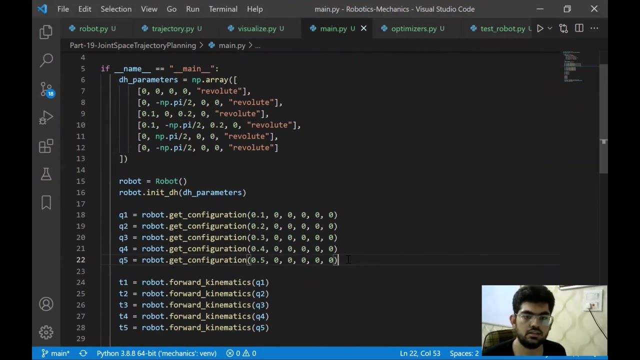 all the errors that we have. so, yeah, all right. so this was a pretty, pretty good learning video as such. so right in the next video. i don't know if we are going to be testing the trajectories- unit testing, since the trajectories are more of a visual component. it is quite 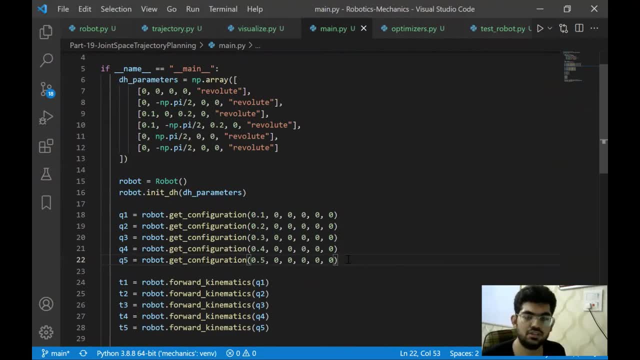 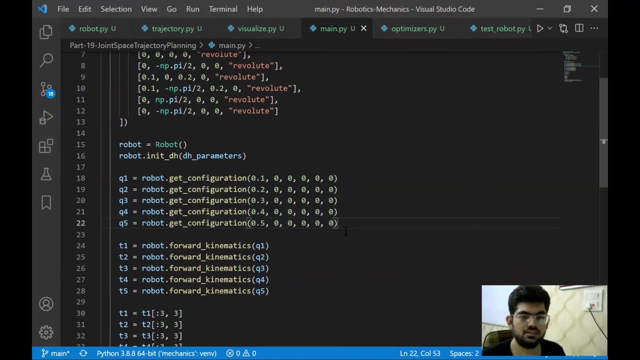 different, It is difficult to execute any unit tests on them as such. so let's see what we get in the next video. like there are some couple of things that we can go. either we can continue with the trajectory planning as such or we can introduce some new concept like controllers. 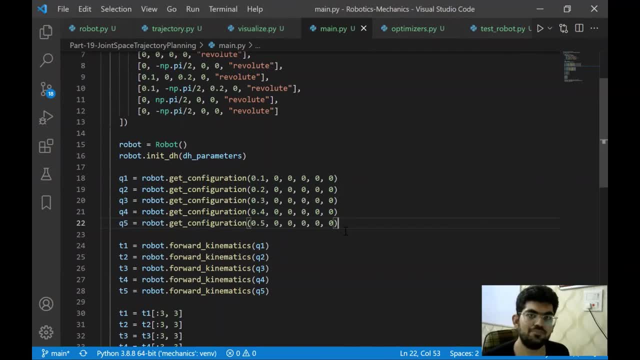 or anything, but let's see what we get in the next video. see you in the next video, then, bye.